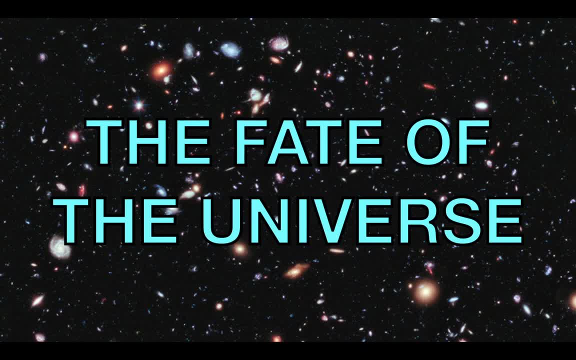 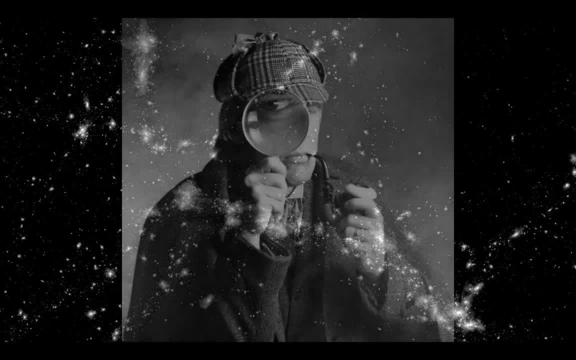 questions as possible, But this is just to make sure that the questions remain non-silly and on topic. Okay, fantastic, Let's crack on. We're learning about the fate of our universe. So, like I said, this is the second part of the. 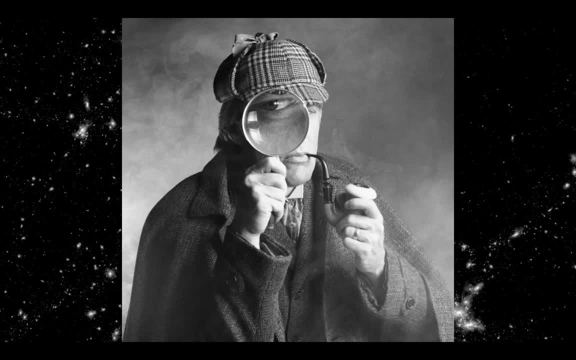 dark universe talk that we started last week. So last week was all about dark matter. This week is about dark energy, which, if anything, is even more mysterious, And it's a big puzzle that we're trying to work out what the future of our universe is. I spoke last week about how 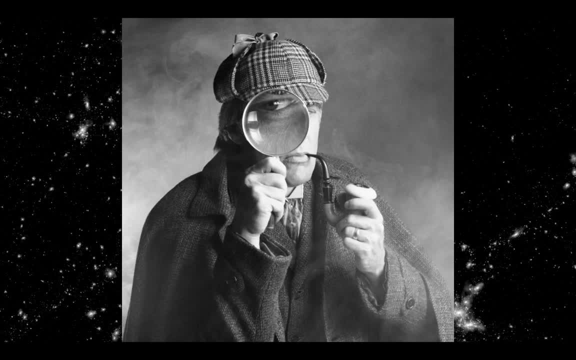 science is a bit like a big detective story- right, It's a scientist, basically detectives of the natural world, where we go out and we try and put together clues to work out what's going on. And this week is no different. We are going and putting together clues to try and work out what 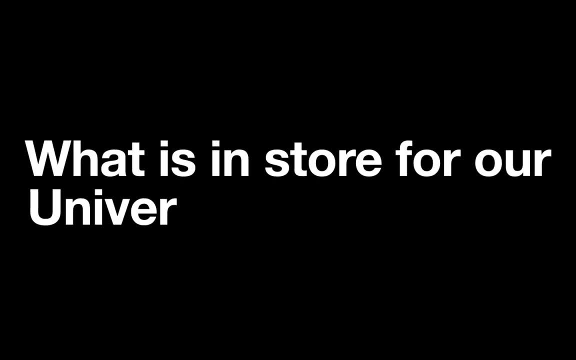 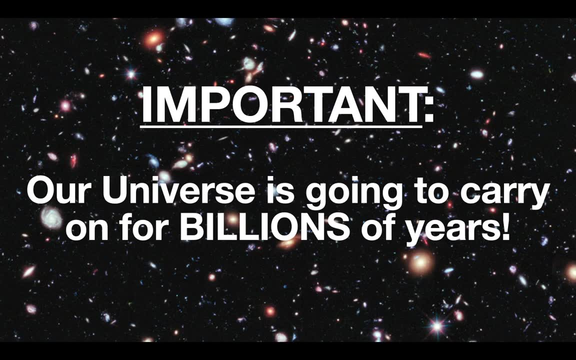 is going to happen to our universe in the future. An important thing to note: our universe is going to live for a very, very long time. So even though this all sounds like kind of doom and gloom, right talking about the end of our universe, I'm not saying the universe is going to end next week. 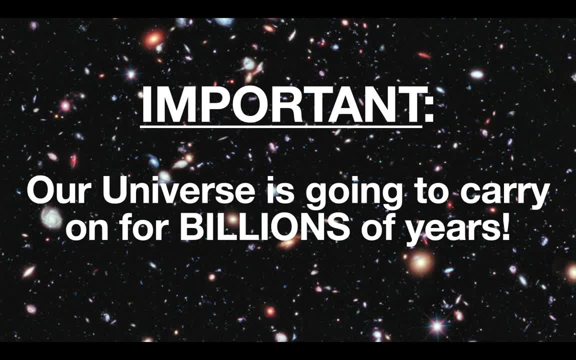 or even next year, or even a billion years from now. Our universe is going to carry on for many, many billions of years to go, So don't worry people out there, Even though we're talking about the end of the universe. 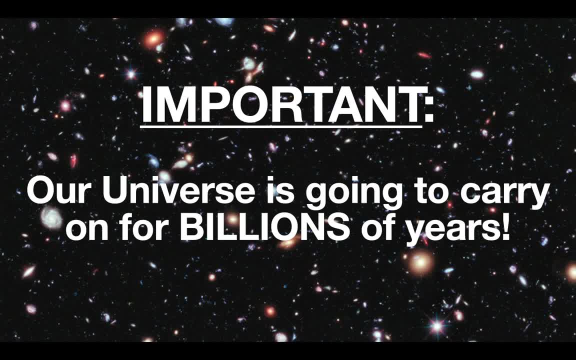 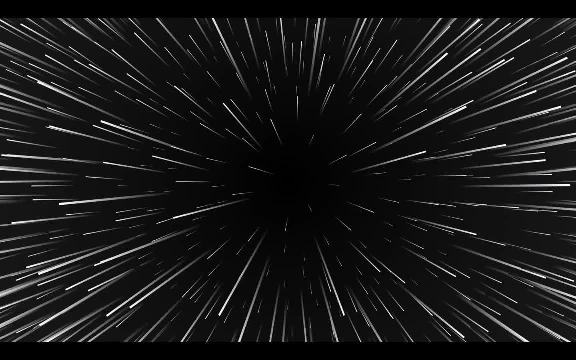 this is really really really far off, distant stuff. The human race. we're absolutely fine for thousands, of millions of years to come, Okay, so have no fear. So before we understand what the future of our universe is going to be, we need to know what. 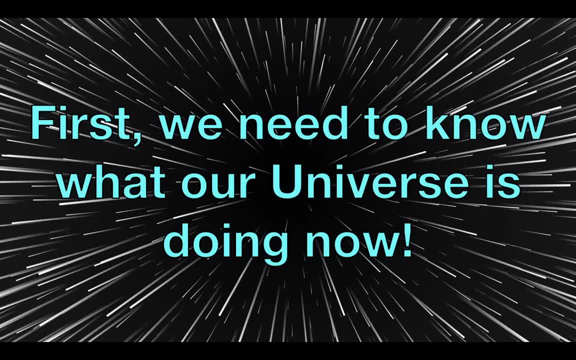 our universe is doing right now, Because if we understand how our universe is behaving at the moment, then we can kind of make predictions into the future and guess what the future of our universe is going to be. So what does our universe look like right now? And so this is a picture. I 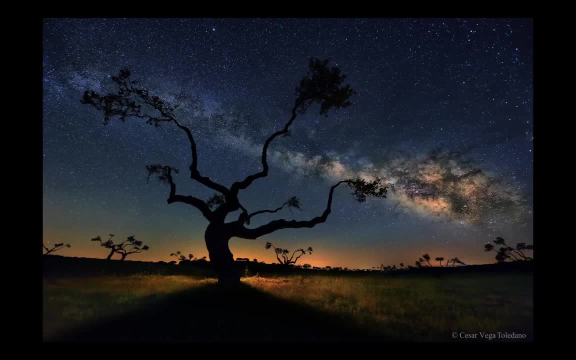 always like showing in astronomy talks because it shows the Milky Way galaxy really nicely. So you can see all kinds of different things in this picture. This is what the night sky looks like if you go out and stand somewhere really, really dark. You can see trees, obviously, but you can 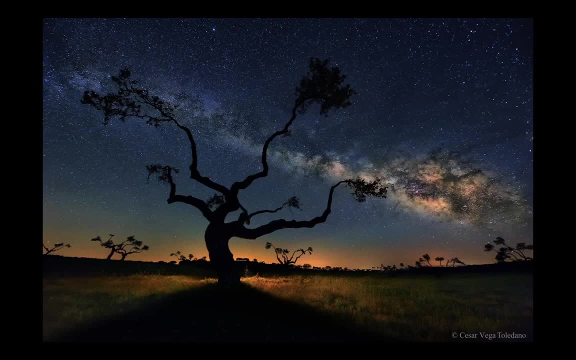 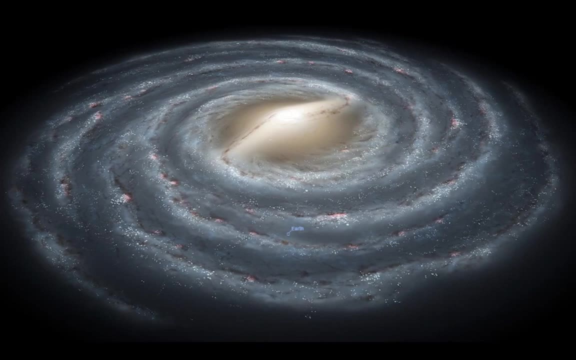 see stars in the sky And you can see the Milky Way galaxy, this nice stripe of light across the sky, And so this is our Milky Way, And this is where I want to start today's talk. So we live in the Milky Way galaxy. our sun is just one of something like 200,000 million stars in our Milky. 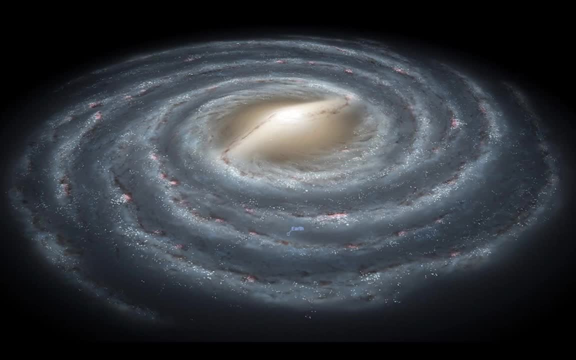 Way, This is something that I spoke about in the first week of these talks right. Our galaxy is 100,000 light years across. It's so big that, even at the speed of light, it would take you 100,000 years to go across it. And the fact that our galaxy is so big, what I'm going to say next? might be not that surprising. In the past, astronomers thought that this is all there was to the universe, And you don't even have to go back very far. If you went back in time 100 years ago and asked astronomers, a lot of them would have said: this is all there is to the universe. 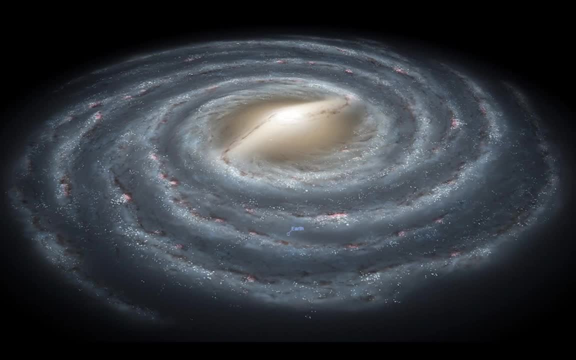 A picture like this that I'm showing you on the screen right now is a picture of everything in the universe. This began to get questioned, right. Astronomers started wondering if there was a universe outside of our Milky Way And the way they settled this. it's really really cool In. 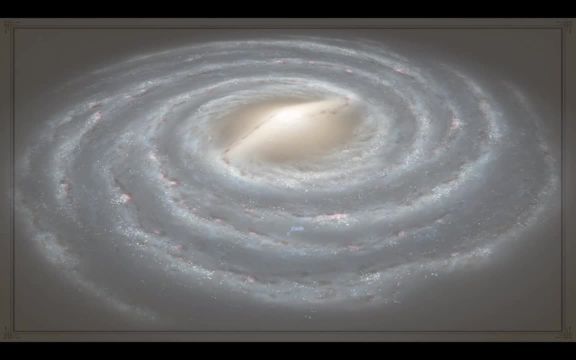 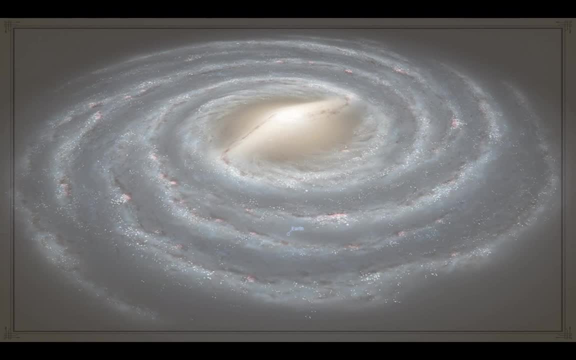 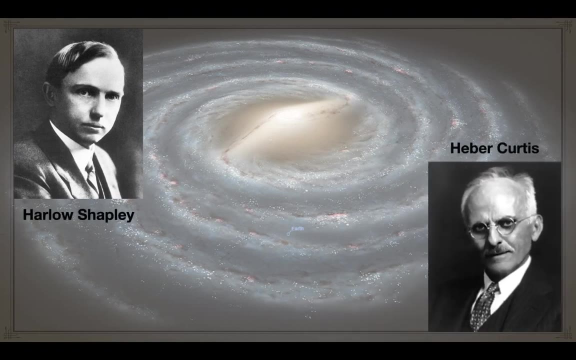 famous debate in astronomy, which is all about whether the Milky Way is the only thing in the universe or whether there's loads of stuff outside as well. And it's between these two guys, Harlow Shapley and Heber Curtis, and who some of you might have heard of, some of you might not. 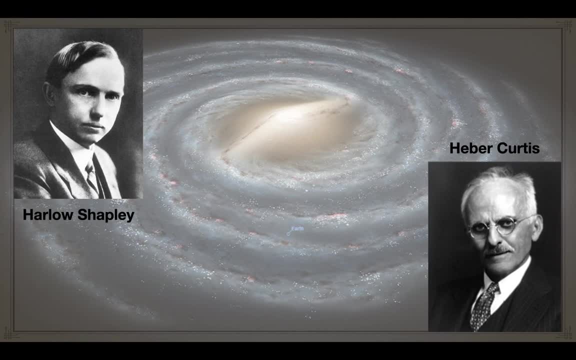 have done. But 100 years ago these two guys were like the top astronomers in the world And they bought tickets right to see these two guys argue this thing out. So Harlow Shapley was arguing for what everyone thought at the time, that the Milky Way is the only thing out there, And Heber 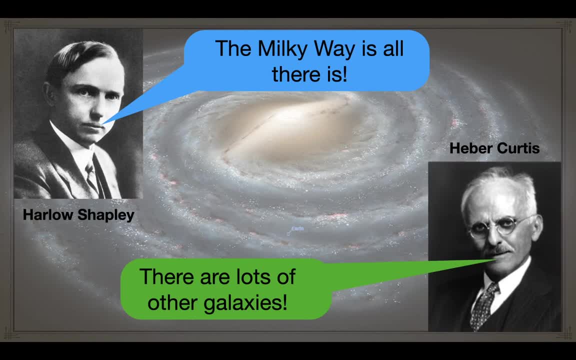 Curtis. this other guy was arguing for this kind of new, exciting idea that there are loads and loads of galaxies and our Milky Way is just one small part of a much, much bigger universe. So we now come to the first of the astronomy quizzes today And I'm hoping this is going to 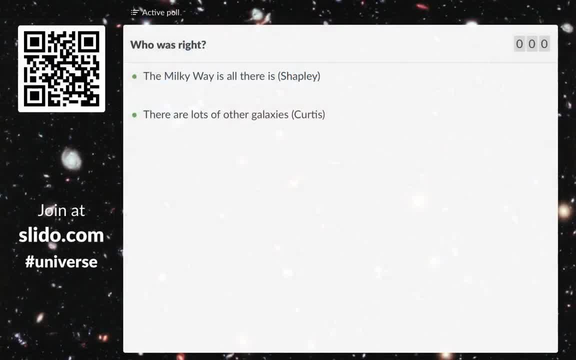 be quite an easy one for you, but we will see. My question to you is: who was right? Was Shapley right? So is the Milky Way all there is in the universe, Or are there loads and loads of other galaxies out there as well? So I'm going to give you a moment to think about this, While 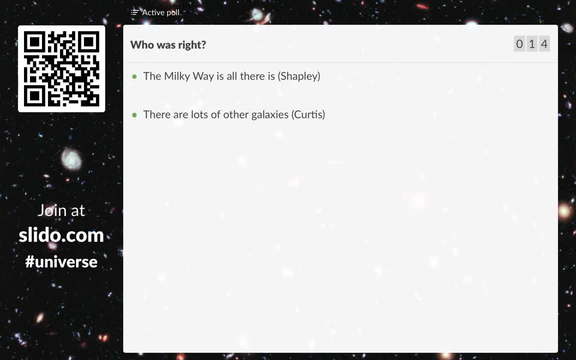 these quizzes are going on. I am going to be trying to moderate some questions, So there's lots of nice questions for our question and answer session at the end. OK, very nice, Just give you a few more moments. OK, let's see what the answer is, And I'm hoping this is going to be quite an easy one to get you. 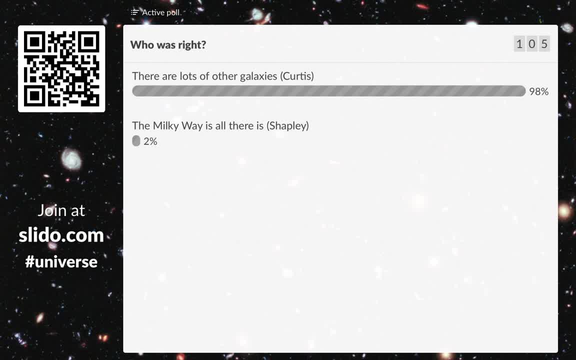 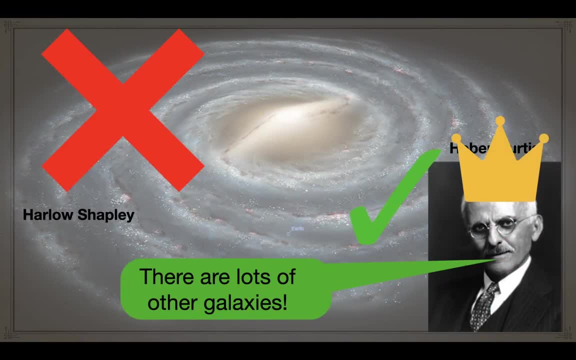 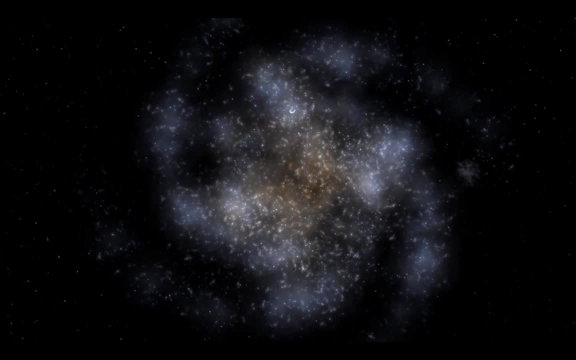 Curtis was right, He yes, and so what he thought about the universe, that the Milky Way is much, much bigger. The universe is much, much bigger than the Milky Way- is completely incorrect. We can actually see this If you go to. there are nice programs. 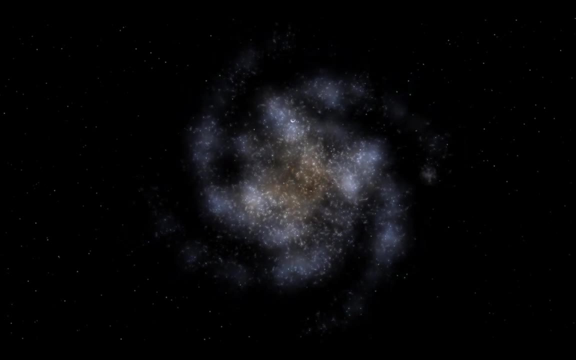 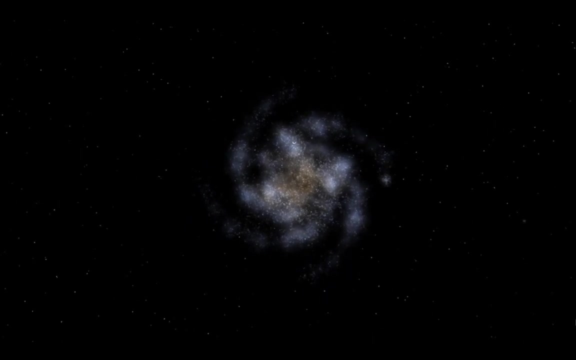 This is a program called Universe Sandbox, which is one that you might like to download and play with. It's a nice thing where you can play with the whole universe, And so we can start with the Milky Way and kind of zoom out to really get an idea of what our Milky Way looks like hanging there in the universe. 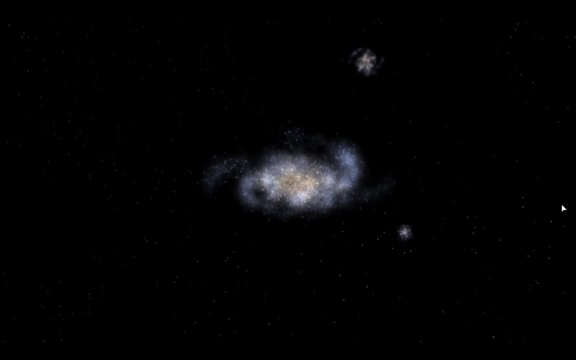 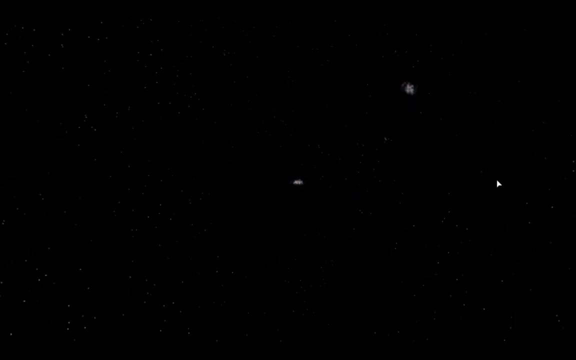 And so this is our Milky Way galaxy, just hanging there all on its own, And we can pan around and see another galaxy. That's the Andromeda galaxy. That's the nearest galaxy to the Milky Way, And if we move this picture around, we can really get a sense of what it actually looks like. 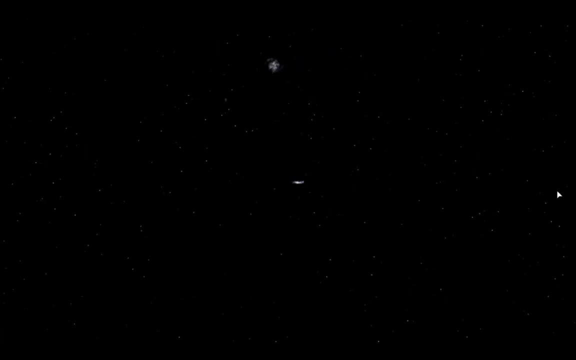 This is the real scale of the Milky Way and the Andromeda galaxy next to each other. So even though the Milky Way is huge, 100,000 light years across it's such a big distance. It really is quite a small part of the rest of our universe. 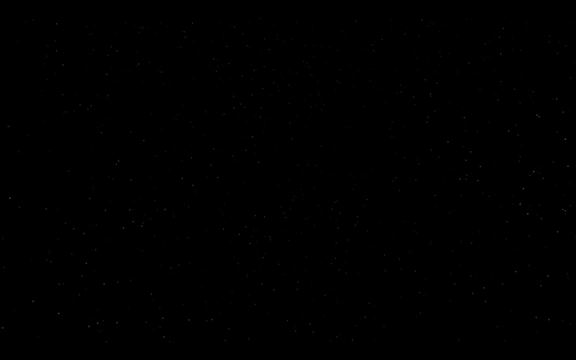 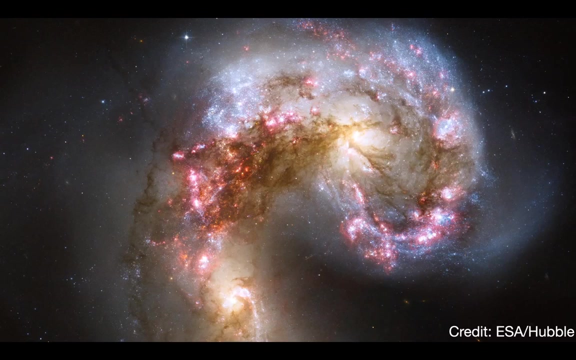 And so, of course, once astronomers discovered that there were lots of other galaxies out there, we wanted to start exploring them and learning about them. So galaxies are some of my favorite things, Right? And so galaxies- are these really, really pretty things in the universe? 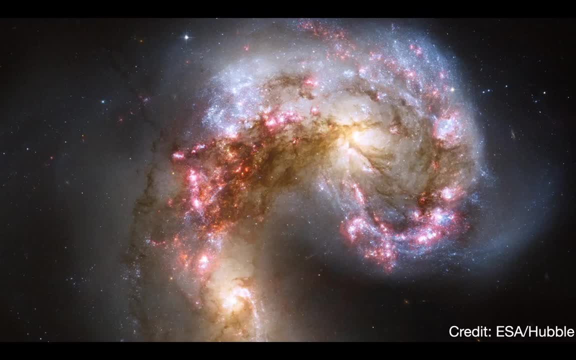 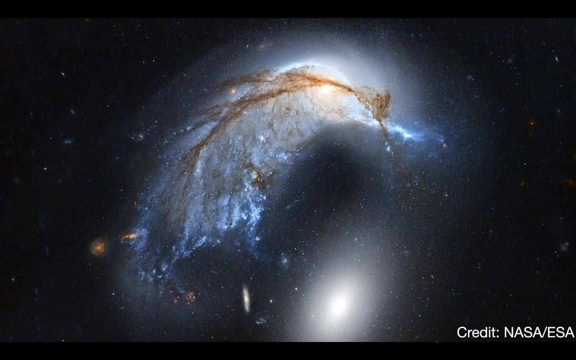 This is one called the Antenna galaxies. It's one of my favorites. This is actually two galaxies crashing together. This is just an excuse to show you some pictures of galaxies. So these are all galaxies, So the things like our Milky Way, but a really, really long way away. 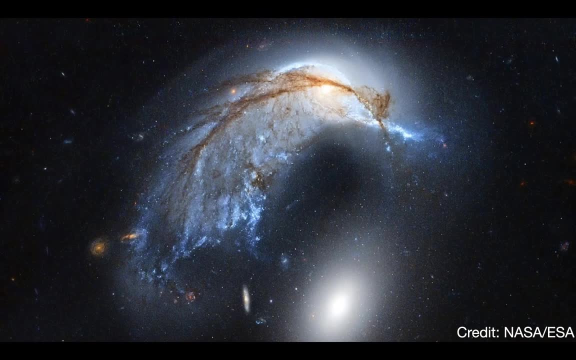 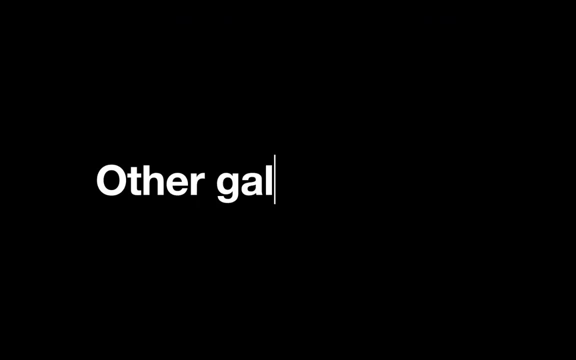 Our universe is full of all of these galaxies, And as soon as we learned that we live in a universe that's full of these galaxies, we wanted to start learning about them. We noticed something Fairly quickly: other galaxies in the universe were doing something quite strange that we didn't expect. 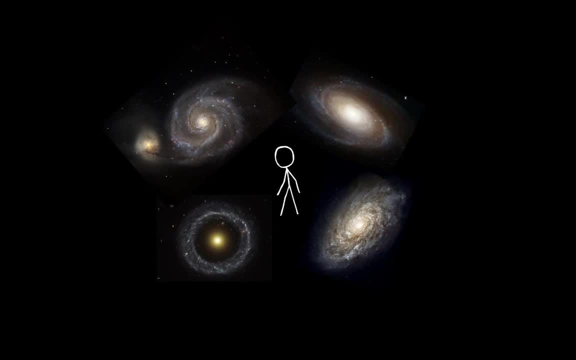 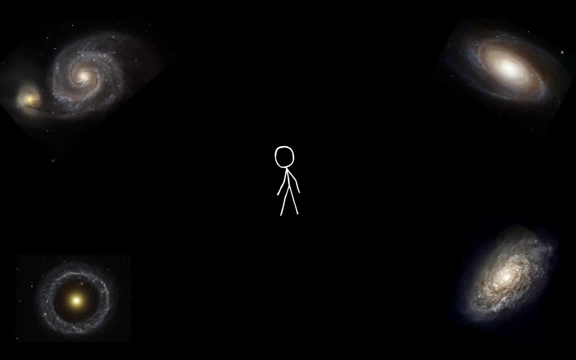 So if this is a, this is a cartoon- right of us in the middle and seeing our other galaxies, what these other galaxies were doing was moving away from us. When we looked all the way around the sky at all different galaxies all across the universe, they were all flying apart. 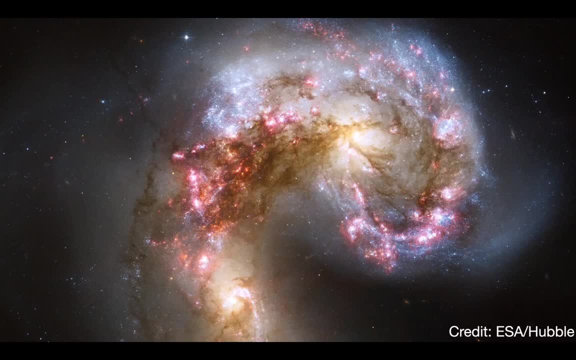 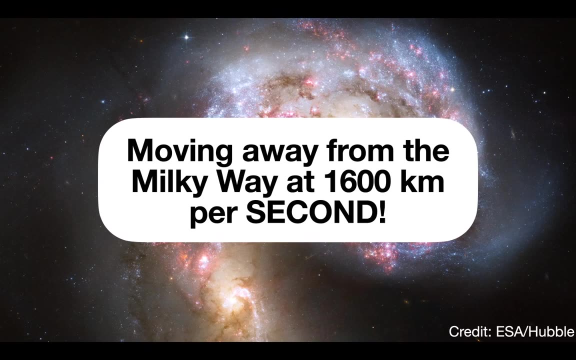 For example, this pretty galaxy I showed you before, The Antenna galaxies. this is moving away from us at the ridiculously large speed of about 1,600 kilometers every second, which I don't know about you. That's almost too much to imagine, right? 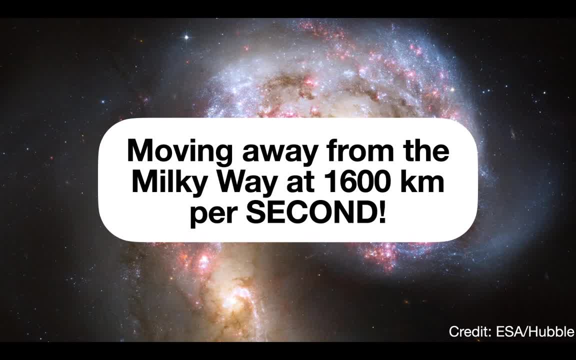 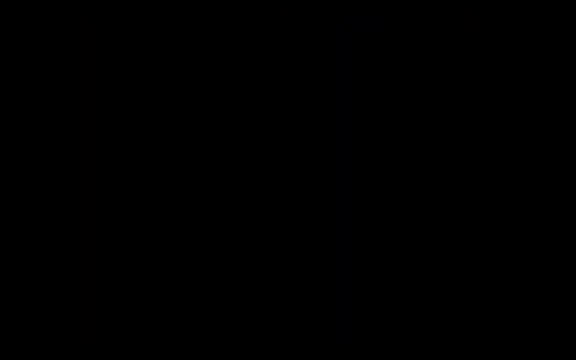 Like 1,600 kilometers per second is a ridiculously fast speed, And this is true of every single galaxy, right? We looked at all these galaxies and they're all flying apart from us, So this was a big surprise, of course, And this is now a very well-known result. 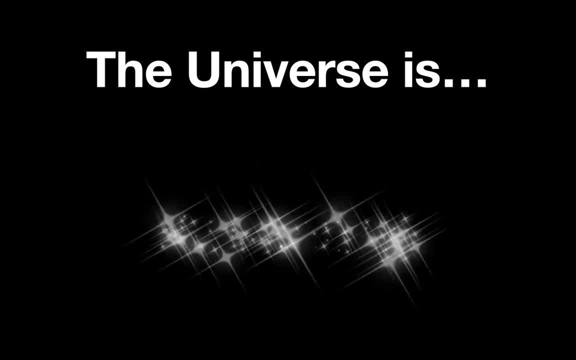 It's one of the most important scientific results of all time. What astronomers found is that the universe is expanding right. That's why galaxies are all moving apart from each other. It's because the universe is growing and growing and growing and getting bigger and bigger and bigger over time. 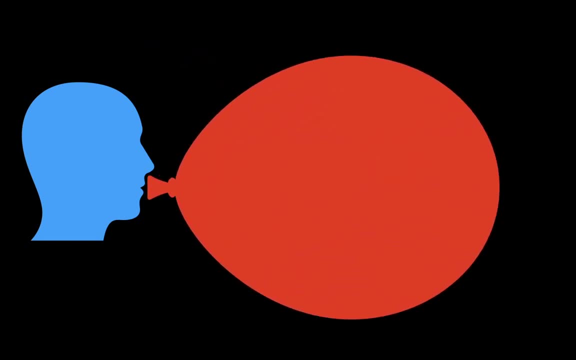 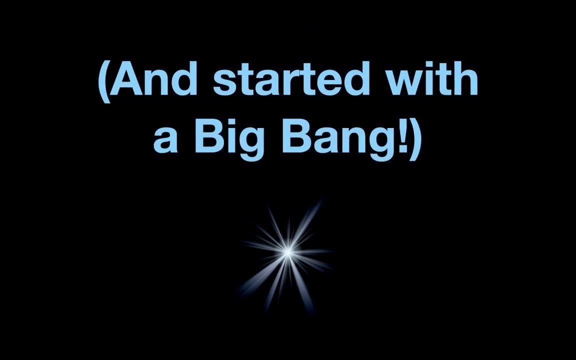 Often, people talk about the universe blowing up like a balloon. right, The universe was small in the past and it's just getting blown up bigger and bigger and bigger. Incidentally, this is how we know that the Big Bang happened, right, Because the universe is getting bigger and bigger and bigger. 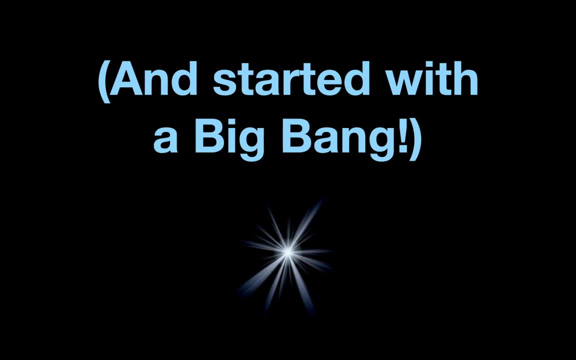 It would make sense that something would have started that, And so a couple of weeks ago, Dr Nina Sartoria, one of the postdocs here, gave a really nice talk, all about the Big Bang, which you can check out on our channel if you want to learn more about the beginning of our universe. 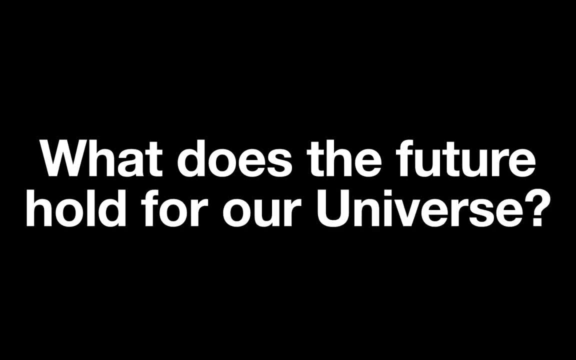 But what? now? we can ask the question. So now we know what the universe is doing. now, right, The universe is expanding. The universe is getting bigger and bigger and bigger. Now we can ask the question: what does the future hold for our universe? 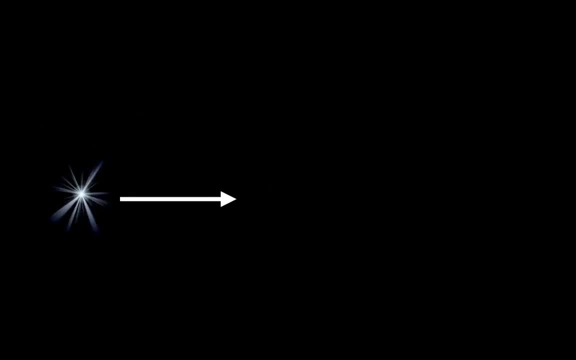 Right, So we start. we know the universe starts with the Big Bang and then some time later, here we are About 13 billion years, Right, 13 billion years later. So what happens in the really really distant future? Now we know that we live in an expanding universe. 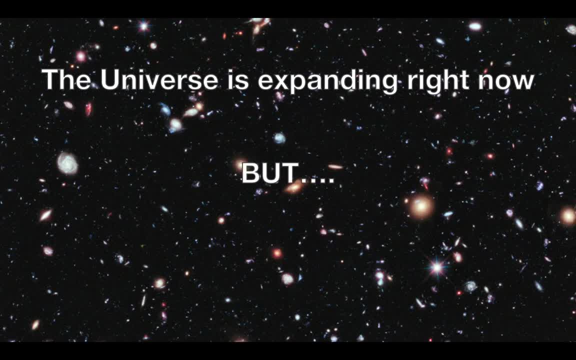 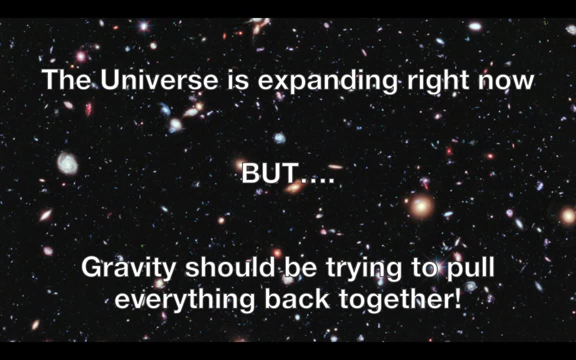 Because, OK, here's the thing to think about. The universe is expanding right now. We know that's true, The universe is getting bigger and bigger and bigger, But we also know that gravity exists. right, Gravity is this force that tries to pull things back together. 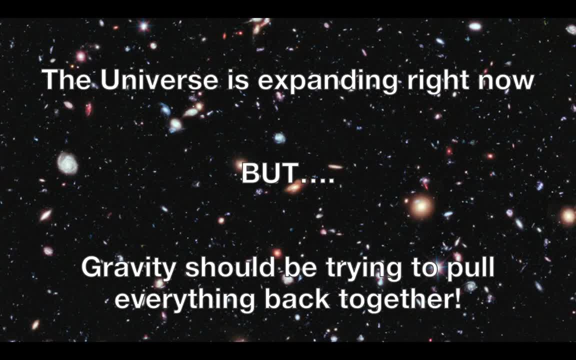 All of these galaxies that are flying apart, gravity should be trying to pull them back together, Right? So maybe one One answer for what is going to happen to the universe in the future is that the gravity is going to try and pull it back together. 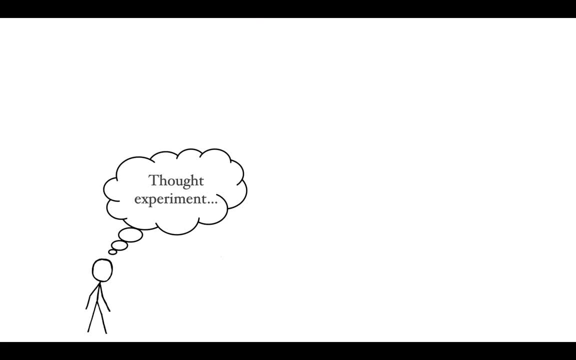 So this gets a bit abstract right, Thinking about what the universe is going to do. And so we're going to do a bit of a thought experiment and kind of imagine what the future of the universe might look like And forget the universe for a moment. 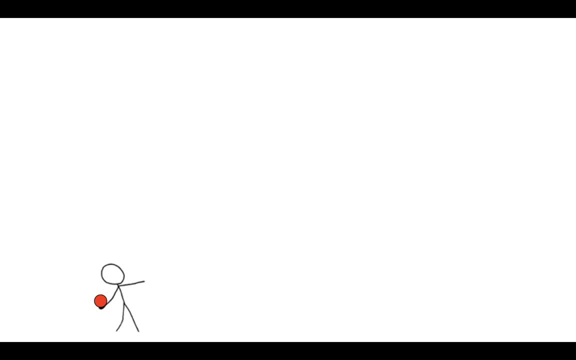 We're going to do an experiment and imagine we are going out into the park and throwing a ball. Now, what happens next depends on how hard you throw the ball Right, And so normally, if you have a normal throw, Like me, the ball is going to do something like this: 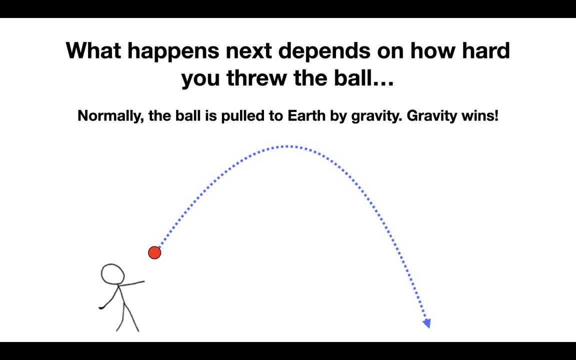 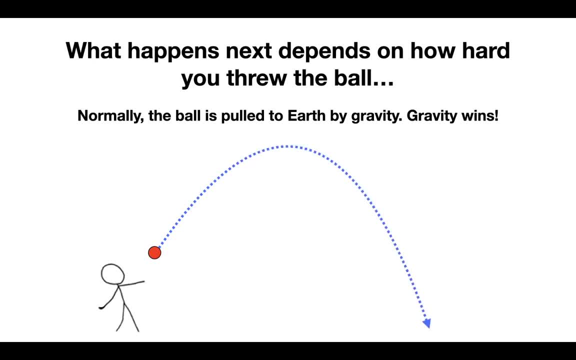 But all the time gravity is pulling on it and gravity is eventually going to beat the strength of my throw and pull the ball back down to Earth. And just to make it clear, like in this analogy, throwing the ball is like the Big Bang. 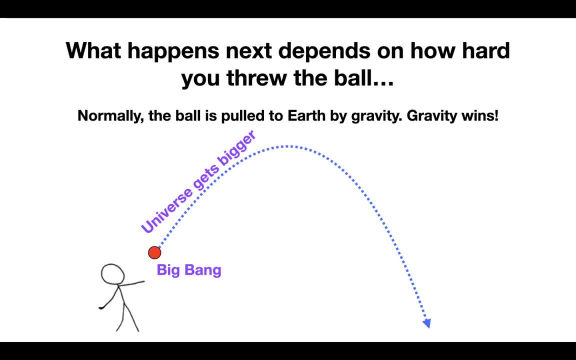 Right. And then the ball getting higher and higher and higher is like the universe getting bigger and bigger and bigger, But eventually gravity wins and the universe gets pulled down smaller and smaller and smaller. So this is one thing that could happen to the universe in the future. 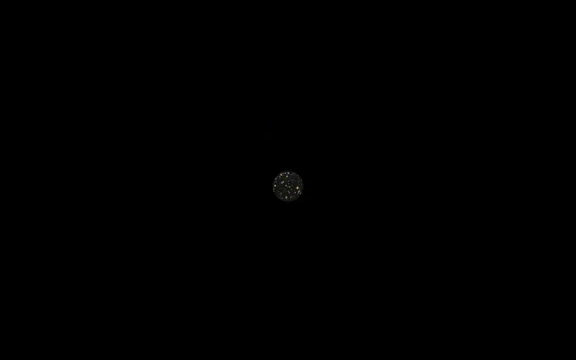 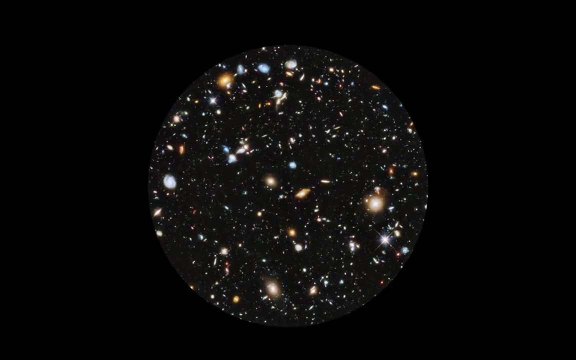 Right, And so this is the idea Right. You start with the Big Bang. The universe is small originally, and then gets bigger and bigger and bigger as the universe expands, But then eventually, gravity wins And then, just like the ball being pulled down to Earth, the universe gets smaller and smaller and smaller again. 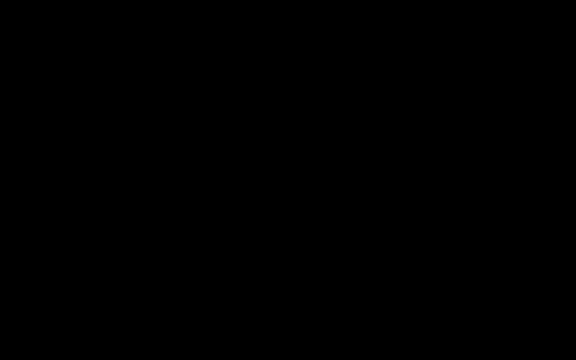 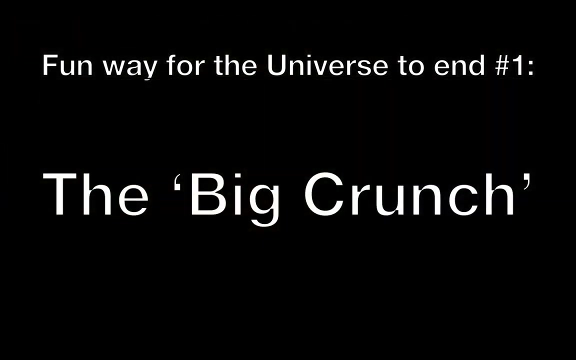 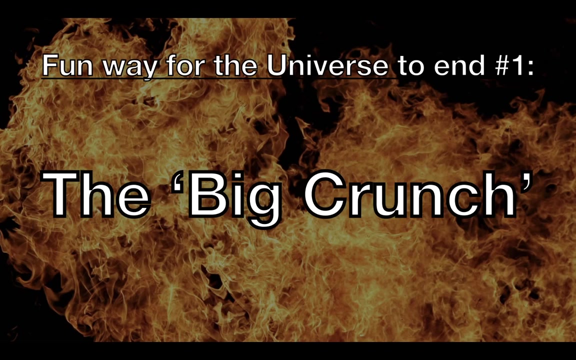 And then kind of does what Crunches down into nothing. And so this leads us to the first of the fun ways that our universe might end, And this is an end of the universe that gets called the Big Crunch. And so this is what happens when the gravity of the universe is enough to pull it back down together. 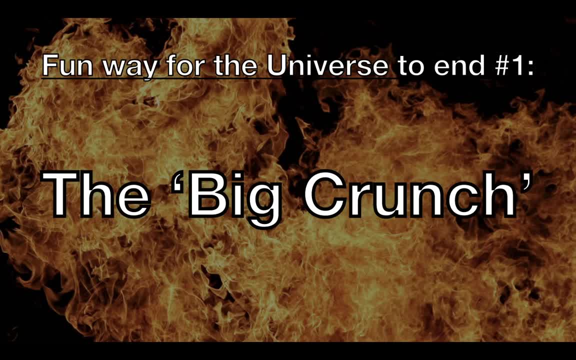 Right. So even though the universe is getting bigger and bigger and bigger right now, in the future, just like a ball being pulled back down to Earth by the Earth's gravity, the universe might get all pulled back together by the universe's gravity. 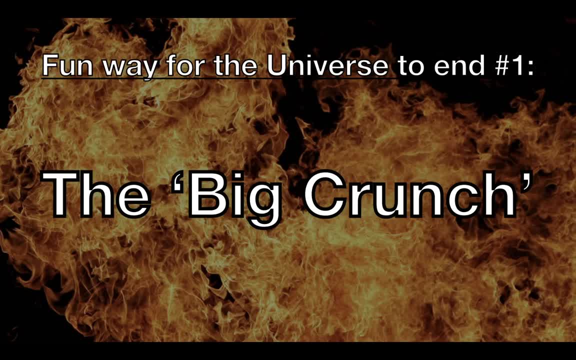 And there'll be something like the opposite of the Big Bang. Right. The Big Bang is the universe starts off small and explodes and gets bigger and bigger and bigger. The Big Crunch is when all the stuff in the universe gets squished down into nothingness. 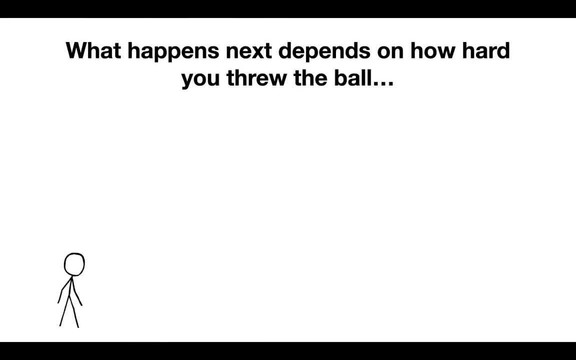 So the Big Crunch is one way that the universe could end, But let's think about something else, Right? So instead of me throwing a ball in the park, imagine you could throw the ball much like far stronger. Say, you're Superman throwing a ball in the park. 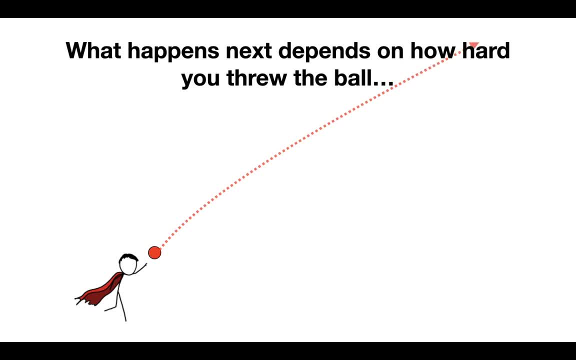 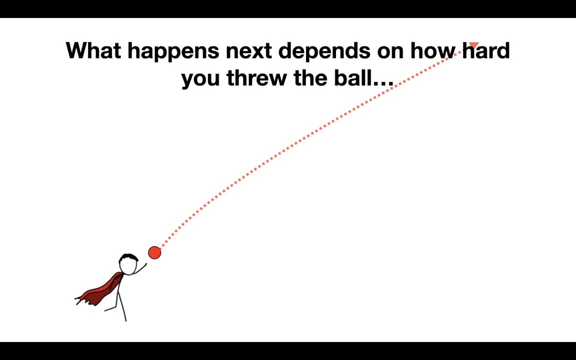 Right, Right, Another potential future for the universe. If gravity is not strong enough to pull the universe back together, then we could have a universe that starts with the Big Bang and then just have a universe that gets bigger and bigger and bigger forever. 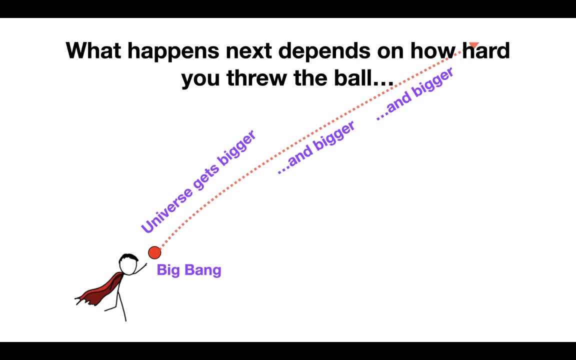 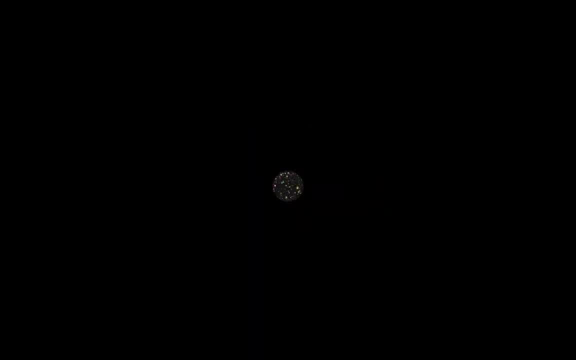 And just like the ball disappearing off into space because gravity couldn't pull it back, the same might happen to the universe. It might just get bigger and bigger and bigger and bigger, because gravity can't pull it down back together. So we know the universe starts with a Big Bang and the universe is getting bigger and 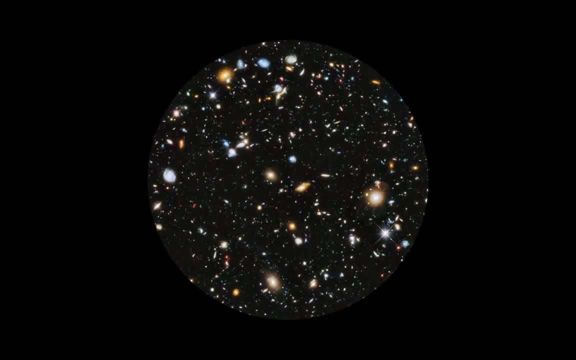 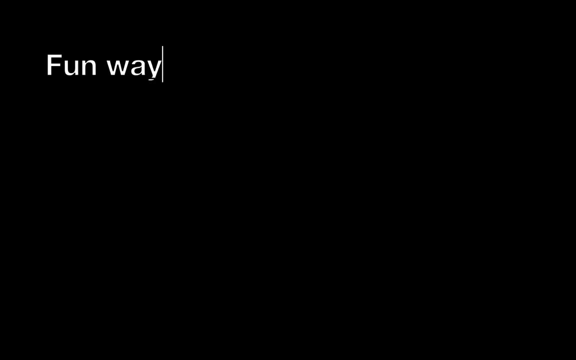 bigger and bigger, and that's what's happening to us now. to us now, but then in the future, the universe will just carry on getting bigger and bigger and bigger and bigger forever. and so this leads us to the second fun way that our universe might end, and 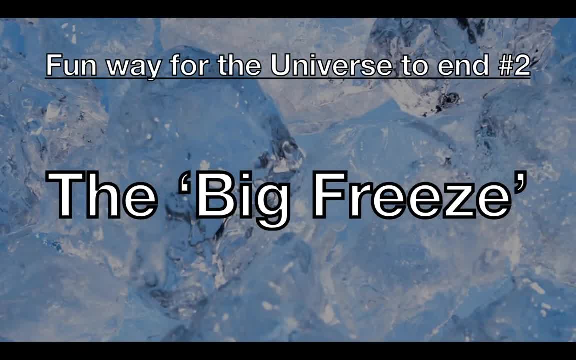 this gets called the big freeze. the reason it gets called the big freeze is because the universe gets bigger and bigger and bigger forever, and it's also going to get colder and colder and colder as all the stuff in the universe gets more and more spread out. so if gravity isn't enough, if the 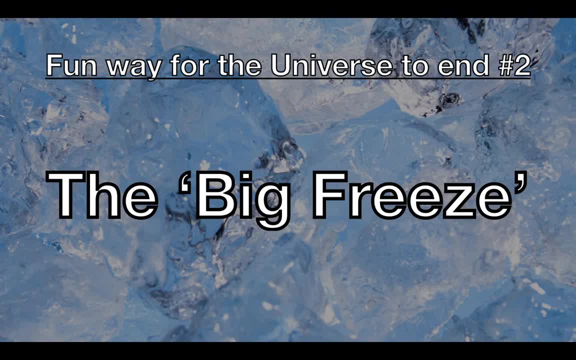 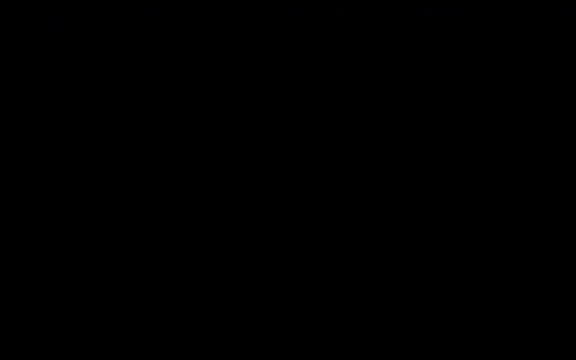 universe doesn't have enough gravity in it to pull it all back together, then, just like, just like superman throwing the wall into space, the universe might get bigger and bigger and bigger forever. so we have this matchup. these are the two possible futures of the universe that we've seen. 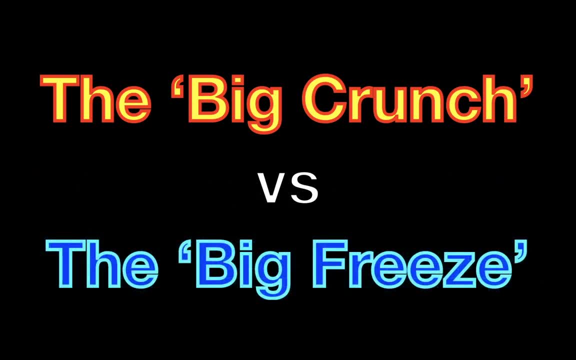 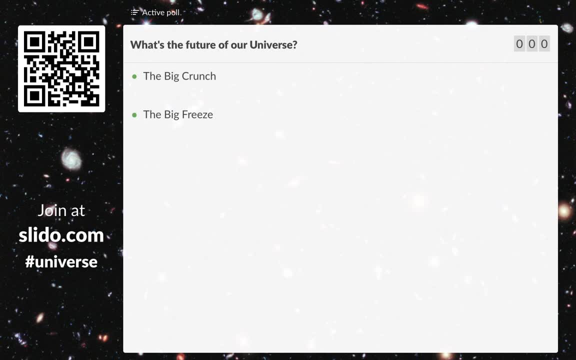 so far, we've got the big crunch versus the big freeze and i want to put it to you. i just want to get a sampling of what you guys are thinking right now. um, there's, yeah, there's- no real right or wrong answer. we're going to carry on and talk more about these things, but i just want to get an. 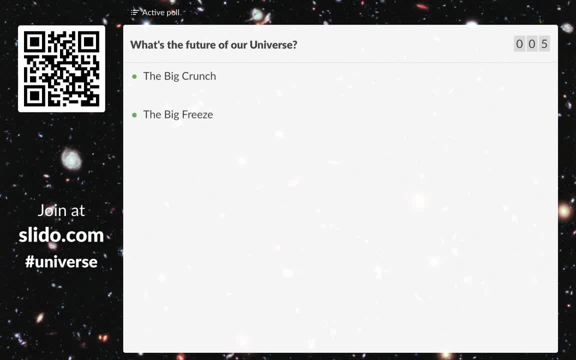 idea of what's going on in the universe and what's going on in the universe and what's going on in what you guys are thinking. do we live in a universe where gravity is going to pull us back for a big crunch or do we live in a universe that, just like superman throwing a ball into space is? 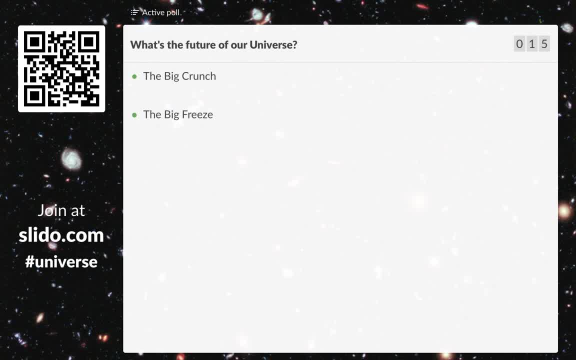 going to beat gravity and get bigger and bigger and bigger forever. and while you are thinking about that, i'm going to moderate some more of your questions. bear with me can see lots of excellent questions coming through, so thank you for doing this. please keep sending your questions in. 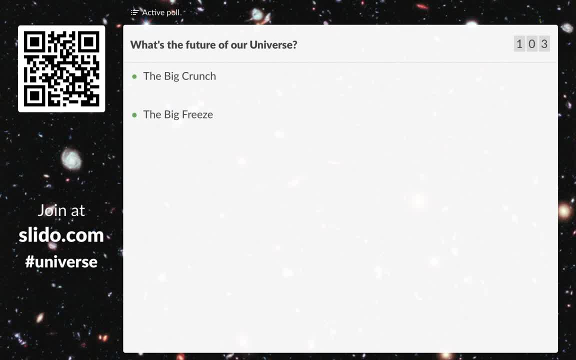 okay, let's just have a look. i want to see what you guys have been saying. this might be a good gauge of how many people are optimists or pessimists. right, maybe, if the people thinking that the universe is going to end in a big crunch, or a bit pessimistic people thinking the big 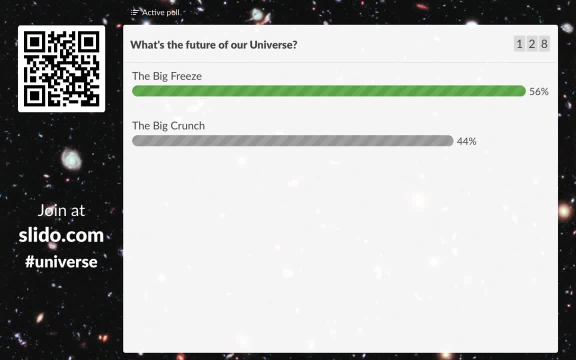 freeze and maybe a bit more optimistic, and it's close to half and half interesting. so slightly more of you, uh, favoring the idea of the big freeze, that the universe will just get bigger and bigger and bigger forever. uh, but about 40 percent of you thinking that the universe is. 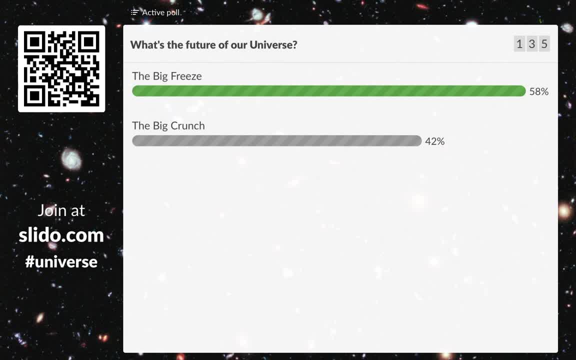 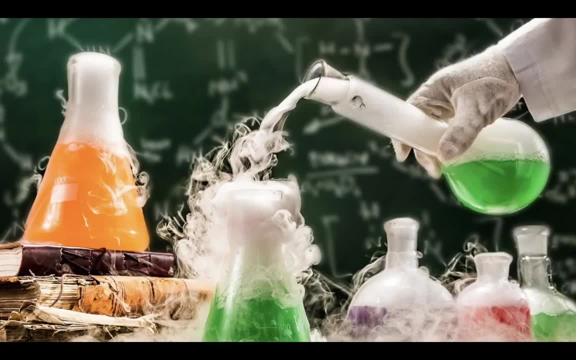 going to end in a big crunch. a gravity always wins, uh type answer: okay, let's go, let's carry on talking and then see, uh, what else we can learn. so you might not be surprised to find out that we did an experiment to find out the answer. right, scientists love doing experiments, and so what we? 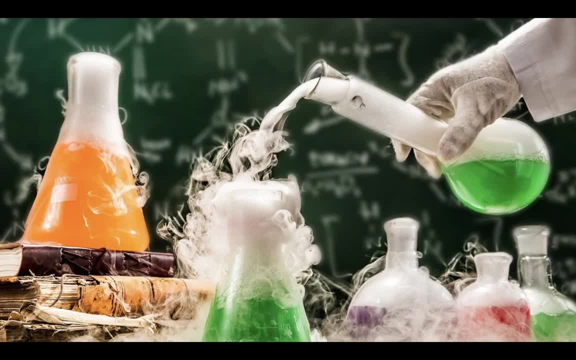 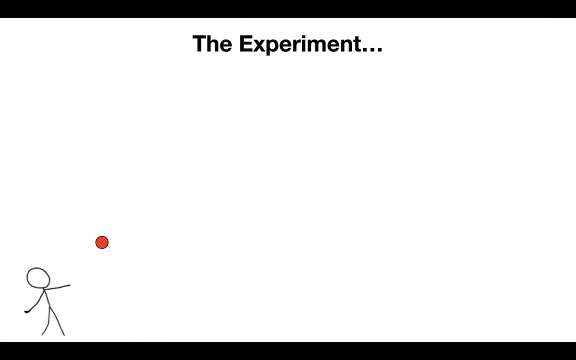 did? we did an experiment to try and learn the answer and to try and teach us whether we lived in a universe heading for a big crunch or whether we live in a universe that can escape gravity and just get bigger and bigger forever. what the experiment is is we basically look at the universe as it is now and try and work out how fast it's expanding. so 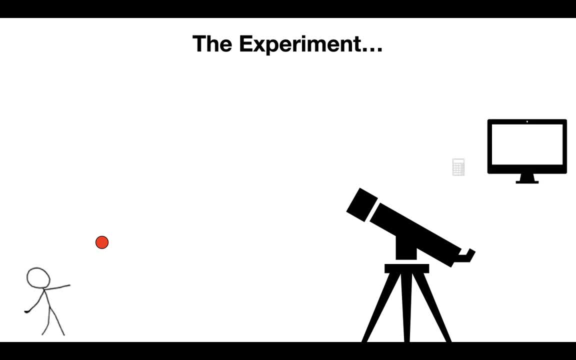 in another way. imagine kind of looking at a photo of someone throwing a ball and then using kind of lots of fancy cameras and computers to work out how fast the ball is going and trying, trying to predict whether it's going to do this and collapse down to the floor or whether it's. 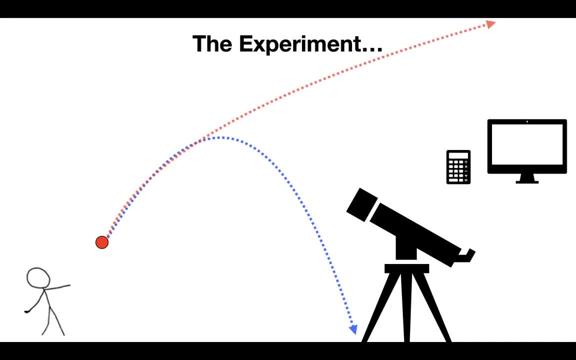 going to disappear off into space. and so what we do? we look all the way around the universe and trying, met and trying to measure how fast the universe is expanding right now and hopefully, if we look carefully enough, that will tell us whether we're heading for a big crunch or whether we're 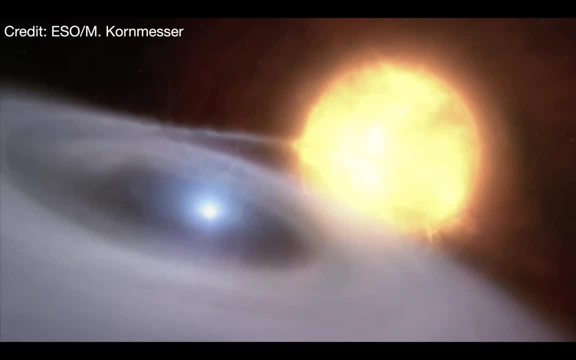 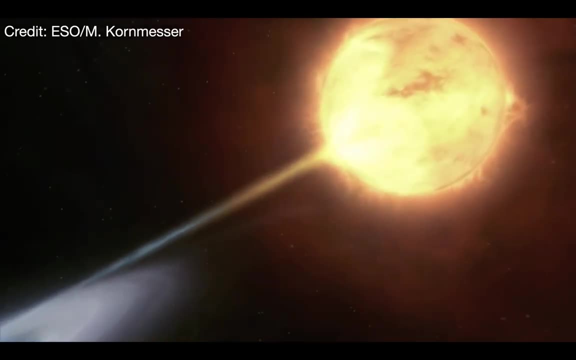 heading for a big freeze. the way we did the experiment is really, really cool. um, so we use these special kinds of exploding stars. so there are these things called white dwarfs that i spoke about back in the stars talk a few weeks ago. white dwarfs can sometimes be orbiting a normal star here. 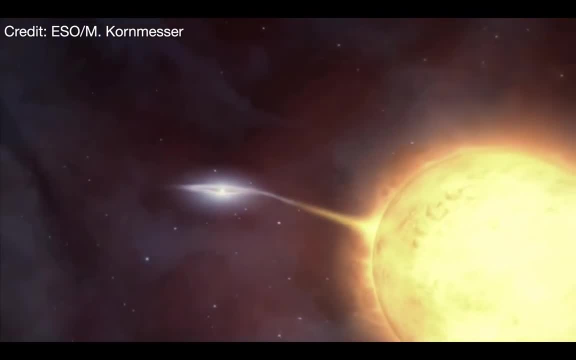 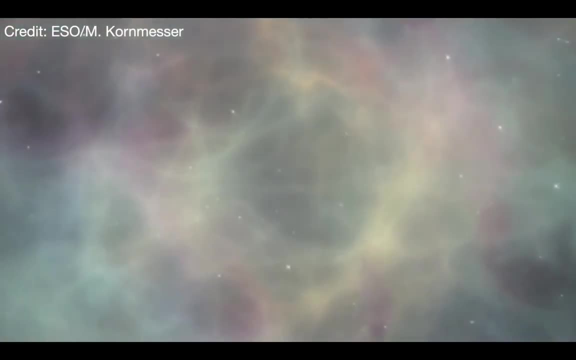 on the right and the white dwarf can kind of gobble up material from the star. and white dwarfs have this weird thing that if they gobble up too much they explode. this they'd explode in this incredible, incredibly violent explosion. and these are really, really useful for astronomers, because when we see 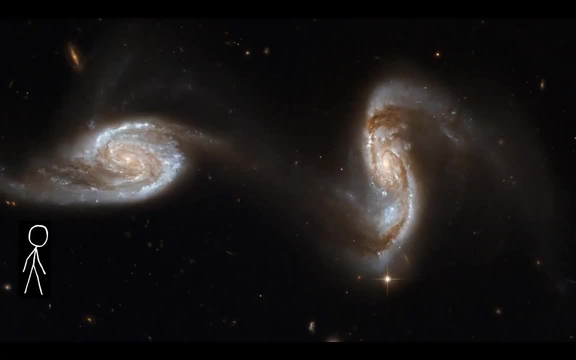 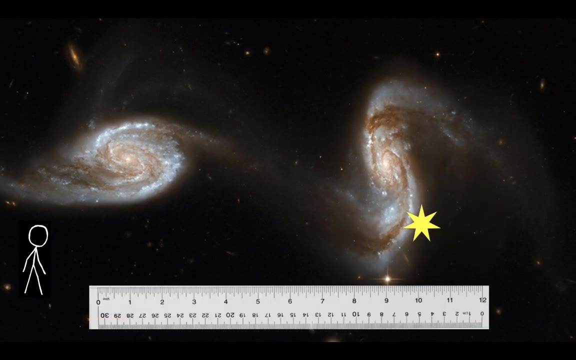 these exploding little stars, we can work out how far they are away. it's really clever. so if we're sitting in one galaxy, in in the next galaxy over we see one of these explosions. that basically lets us use a cosmic ruler if you like to work out how far that galaxy is away. so all we have to do is 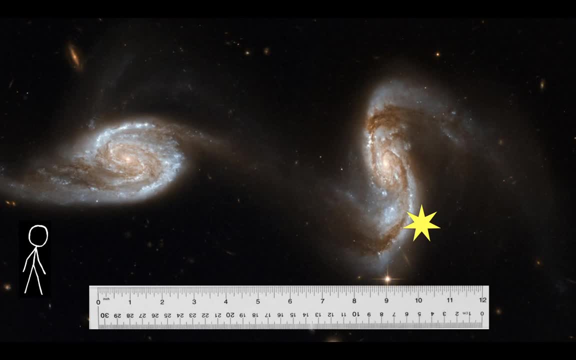 just look at loads of these exploding stars all the way around the universe and that will give us the answer to the experiment. it will tell us whether we're heading for a big crunch or whether we're going to disappear off and expand forever, because we were able to work out how fast the 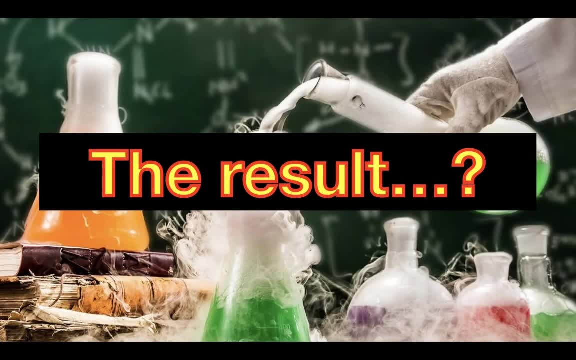 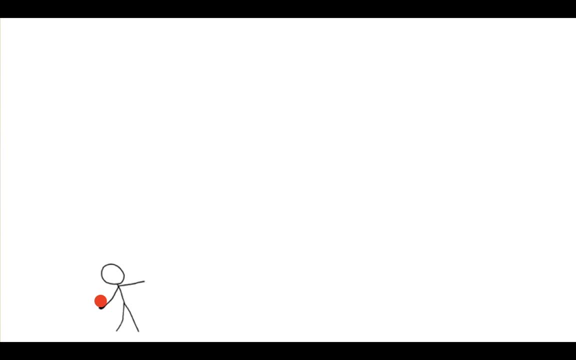 universe is growing right now. so what's the answer? what is the result of the experiment? um, I will tell you the result in terms of throwing the ball in the park, right, because this makes it a little bit easier to understand. I want you to imagine that you've gone out into 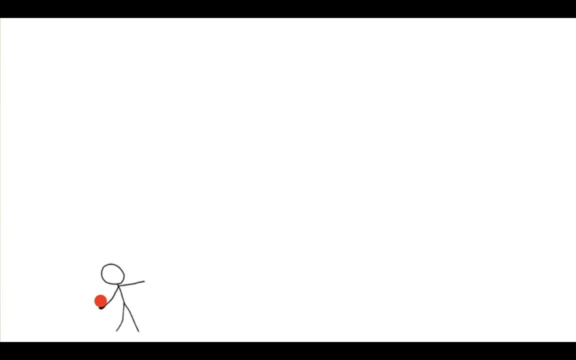 the park and you've thrown a ball in the air, but instead of flying, but instead of coming back to the air, the ball goes flying faster and faster and faster and whooshes off up into the clouds that, if that happened to me, that would be one of the most bizarre and surprising things that had. 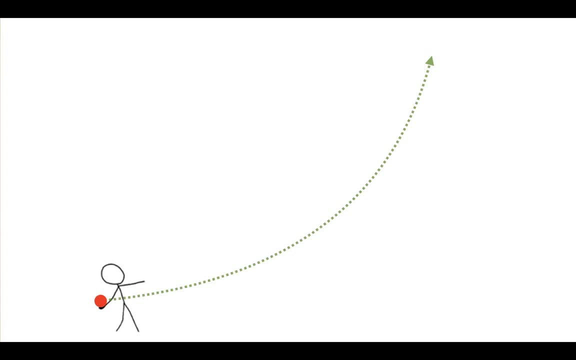 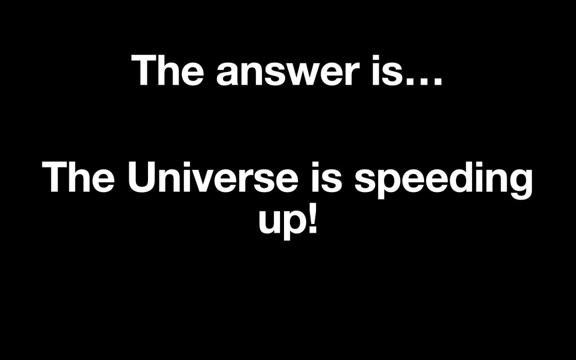 ever happened. right, but this is what's happening to the universe- the universe also. the answer to the experiment is that the universe seems to be speeding up. right, remember we thought gravity should be pulling it back together. it's actually the opposite, is true: the universe seems to be. 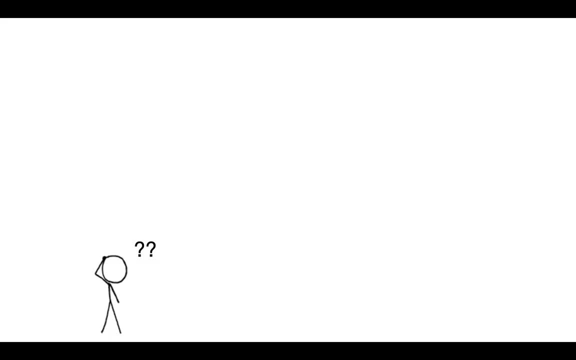 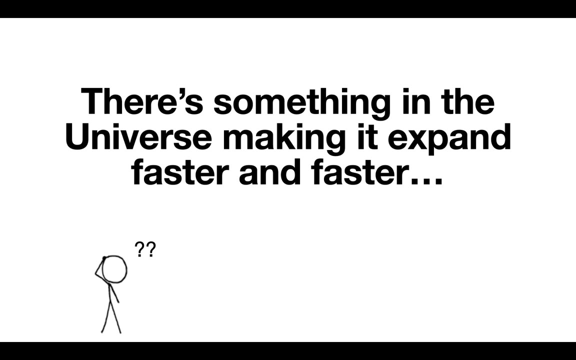 expanding faster and faster and faster. so this really is just like throwing a ball in the air faster and faster until it whooshes off through the clouds. that if, yeah, that would be the most bizarre thing I ever saw, and so we know that there is something in the universe that is making it. 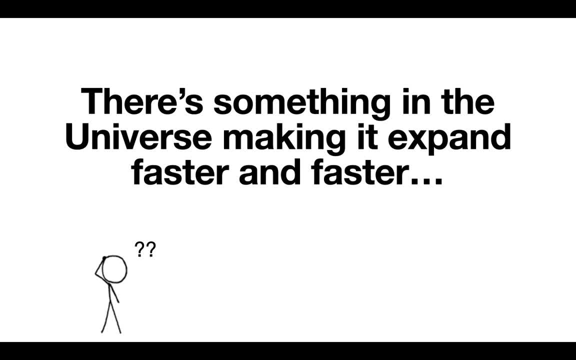 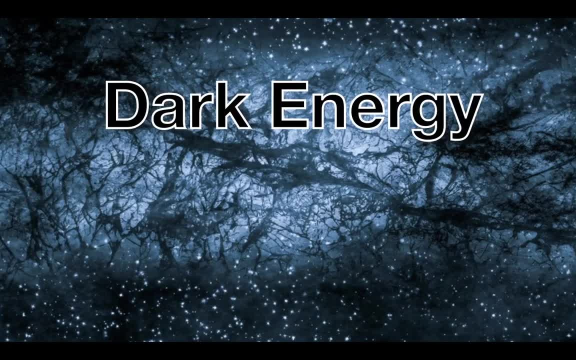 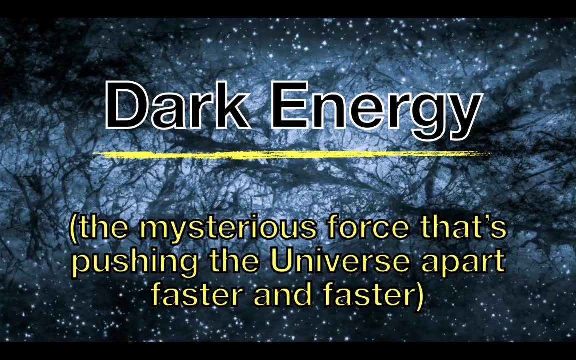 expand faster and faster and faster. there's something that seems to be pushing the universe apart faster and faster and faster, so we call this thing dark energy, and so dark energy. we don't really know what it is, it's just the name that we give to this mysterious Force that seems to 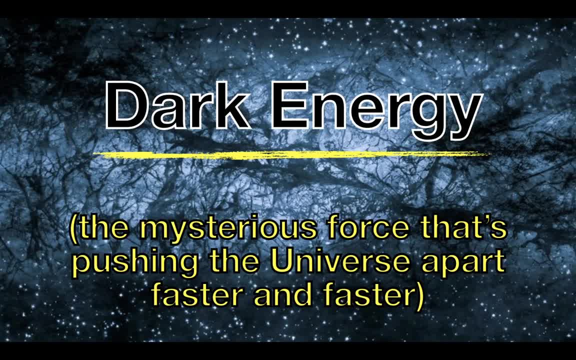 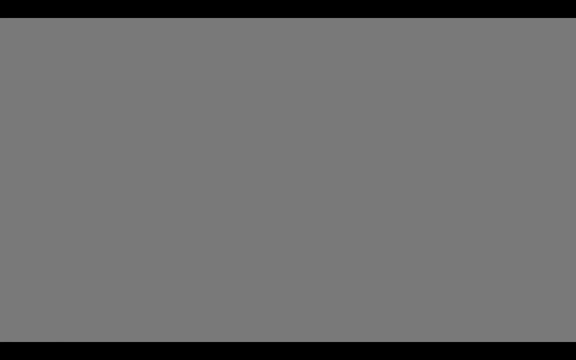 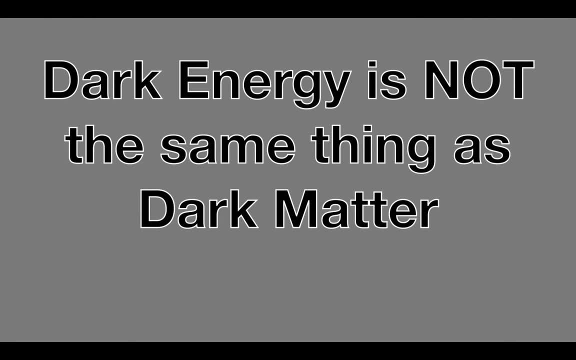 be pushing the universe apart and speeding up the rate that the universe is expanding, right. so dark energy is this stuff that we see that is pushing the universe apart faster and faster and faster. a really important note. just a quick side note: dark energy is not the same thing as dark matter. this confuses loads of people. it's a 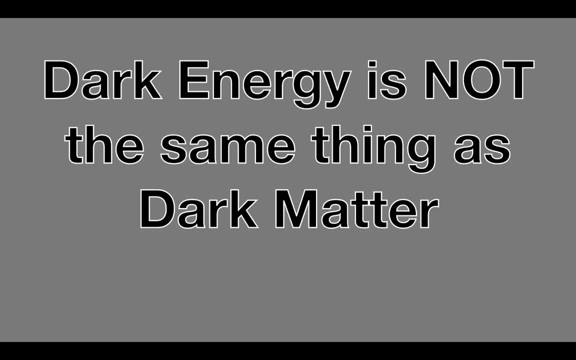 totally reasonable mistake to make, because they sound kind of similar. right dark energy, dark matter. the only thing they have in common is that they have dark in their name, and what we mean by dark is we can't see them, right. so dark matter is this kind of invisible matter. 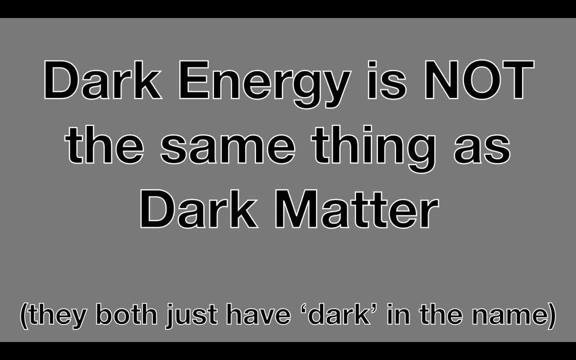 that seems to be all the way through the universe. so we spoke about that last week. dark energy is this kind of invisible stuff that seems to be pushing the universe apart. but don't be confused by the fact that they both have dark in their name. they're completely. 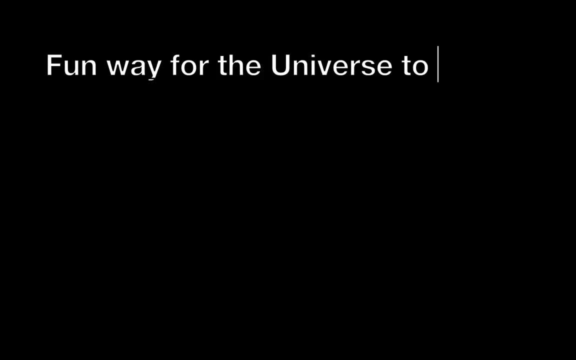 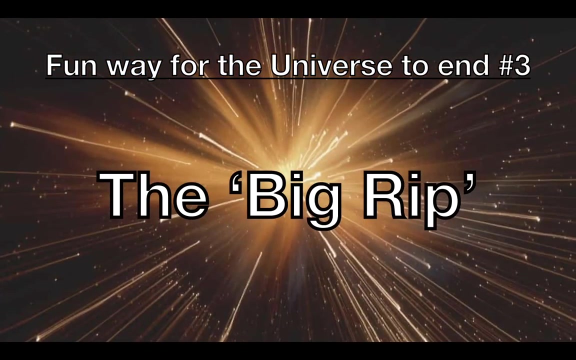 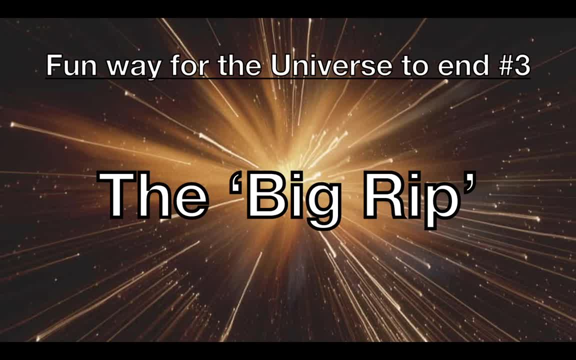 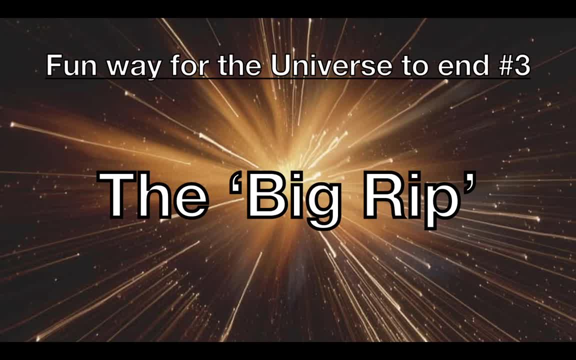 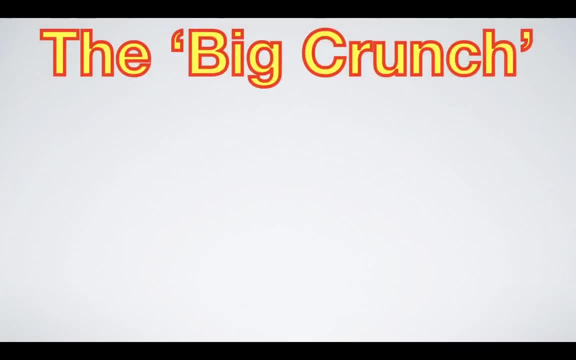 and eventually it would just go get so big, so fast it tears itself to pieces, and this gets called the big rip. and so now we have these. we have a three-way matchup for the future of the universe. we have a big crunch where gravity wins, and we have a big freeze where gravity doesn't win and the universe just. 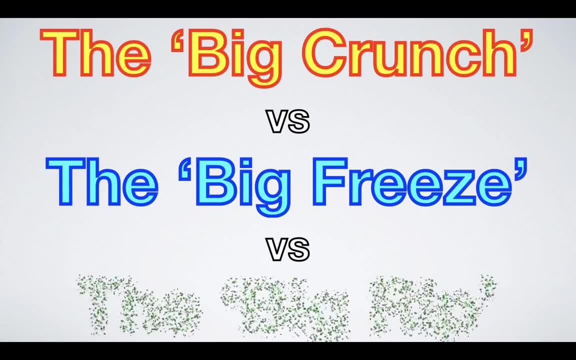 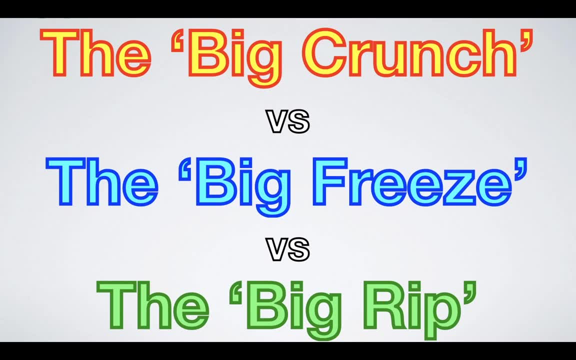 happily gets bigger and bigger forever. and we also have the big rip where maybe dark energy can make the universe go faster and faster and faster and eventually just get too big, too fast and tear itself to pieces. so i'm going to ask you the same question again: uh, what the future of our 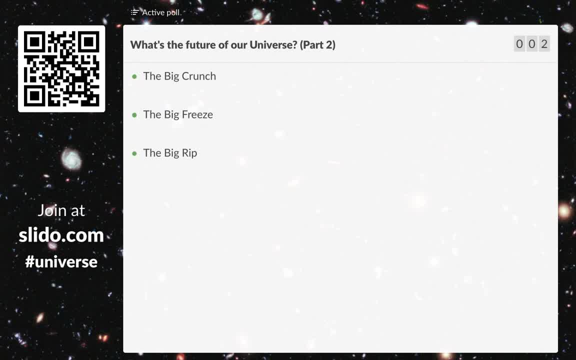 universe. do you think it, might be given that we know that dark energy exists? okay, so have a think about that one for a moment. you can see lots of really fantastic questions coming in. i feel like i should play the countdown music or something to kind of accompany this thinking. 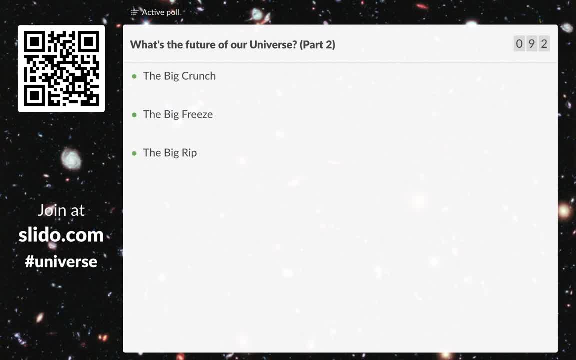 okay, just give you a few more moments. okay, let's have a look at what you guys are saying. okay, so the big crunch has massively lost popularity. uh, the big rip is the winner? fully 70 of you having the very cheerful thought that the universe might tear itself to pieces, uh, in the future. um, let's go back to the 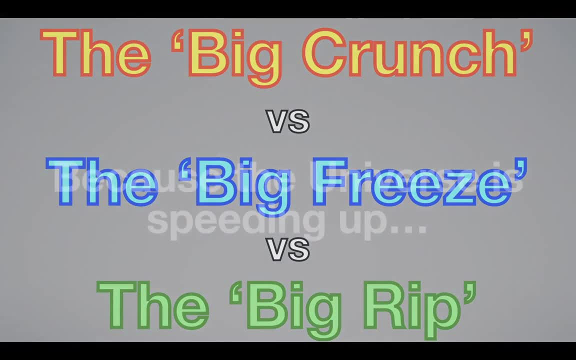 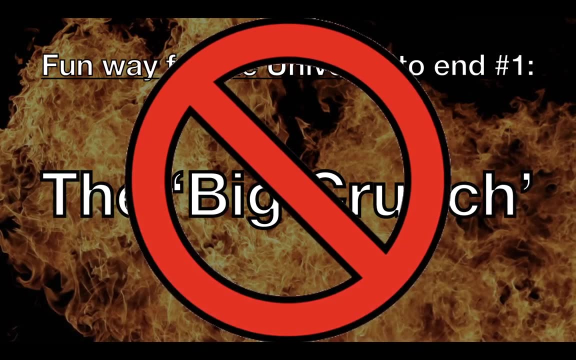 presentation. let's say that's very interesting. let's go back and have a look. um so as, as lots of you kind of guessed correctly, because the universe is speeding up, the big crunch is not that likely, right? so the big crunch was the idea that gravity might win. 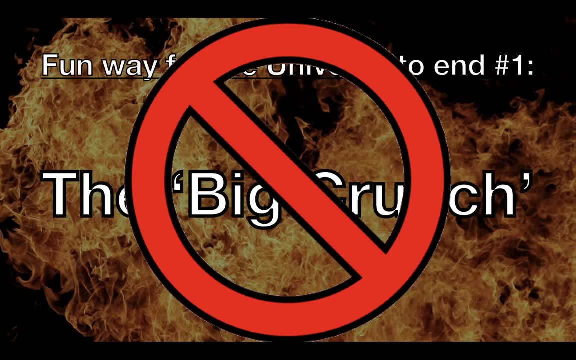 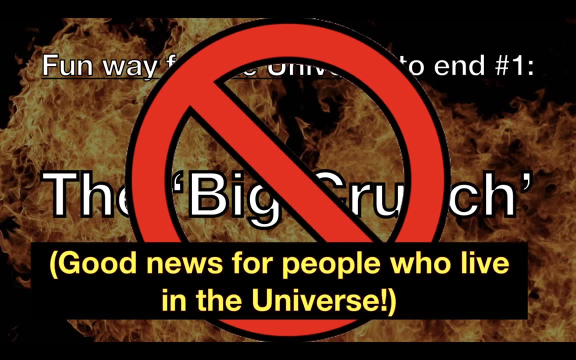 and squish the universe back down to nothing. given that there seems to be this weird stuff in the universe pushing it apart faster and faster and faster, the big crunch is probably going to win at least the biggest part of the table, which is kind of good news. if you, if you. 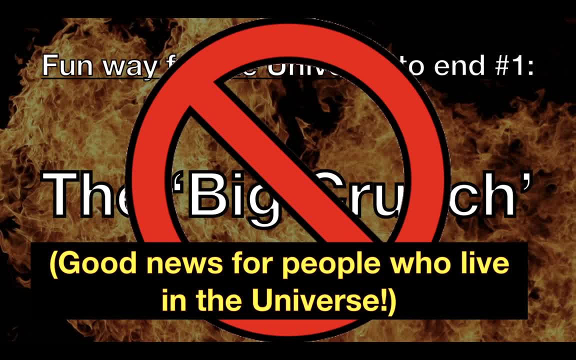 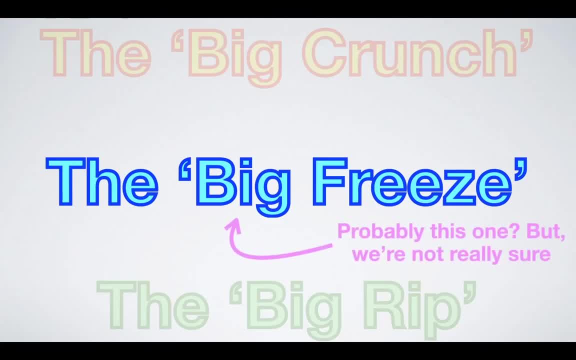 are someone who lives in a universe which i'm guessing that everyone listening is, and this is good news. it means our universe is not going to be squished down to nothingness, which is a reason to be very cheerful. um, i'll say, i'll say here we don't actually know the answer for sure. um, i think. 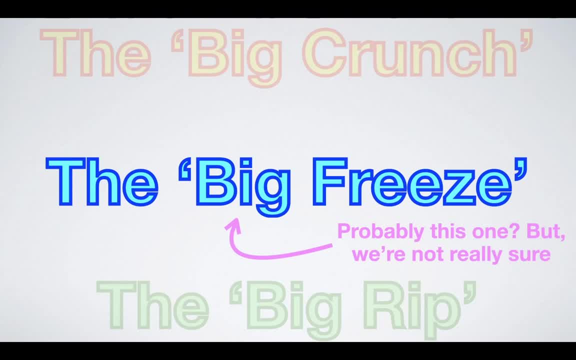 the most likely, the most popular guess is that the universe is going to end in something called the big freeze. so the best, our best guess is that the universe is just going to get bigger and bigger and bigger forever. But I will say we're not sure. 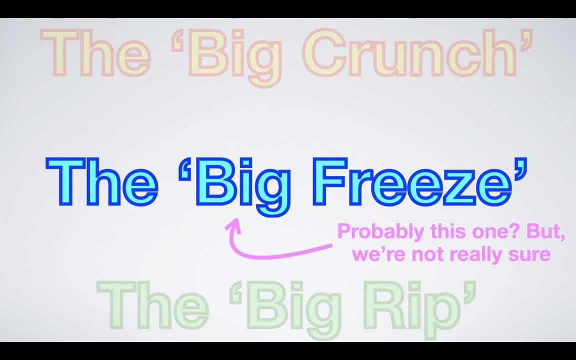 There are some people think that's the big rip might happen. There are some people that think the big freeze might happen As of right now. it's a bit of a mystery, But the big freeze is our best guess, Which is, if you think about it, it's almost a happy ending, right. 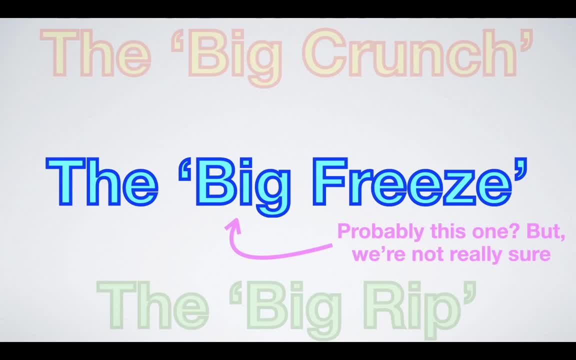 It just means our universe gets to get bigger and bigger and bigger and bigger forever. It doesn't crash down to nothingness, It doesn't tear itself apart. Our universe just gets to go on forever getting bigger and bigger and bigger. So I think that's the most cheerful of the possible universe futures. 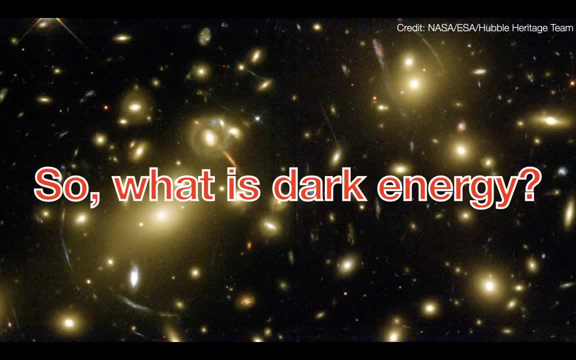 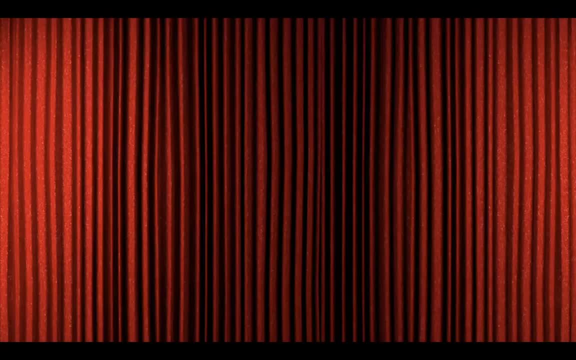 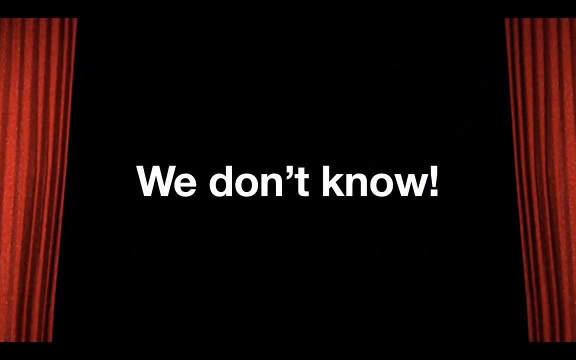 So what actually is dark energy? I keep on saying this mysterious stuff that's pushing the universe apart faster and faster and faster. What actually is it? And the answer is pretty similar to the answer I gave for dark matter last week. We don't really know. 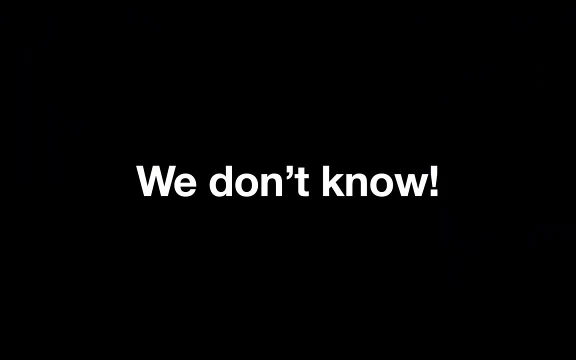 Dark energy is a mystery. If anything, it's even more of a mystery than dark matter. At least, with dark matter we have an idea that it's a particle, probably, that is kind of around and we just don't see it. But dark energy, it's a mystery. 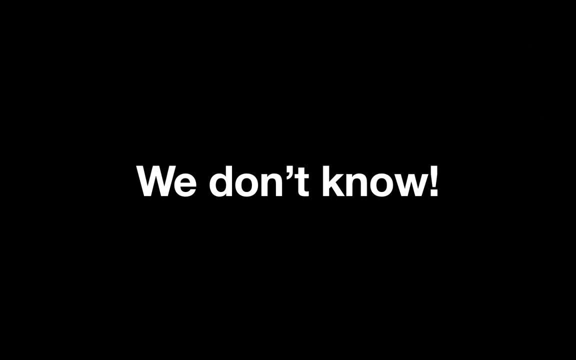 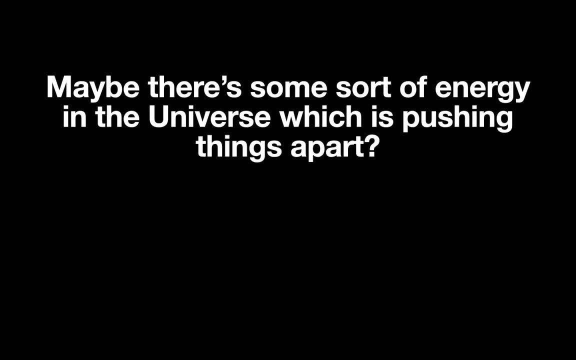 We see the effect of it because we can see the universe getting pushed apart faster and faster and faster, But what it actually is is a real mystery. There are some different ideas. So one idea is that there's some kind of energy in the universe that is pushing things apart. 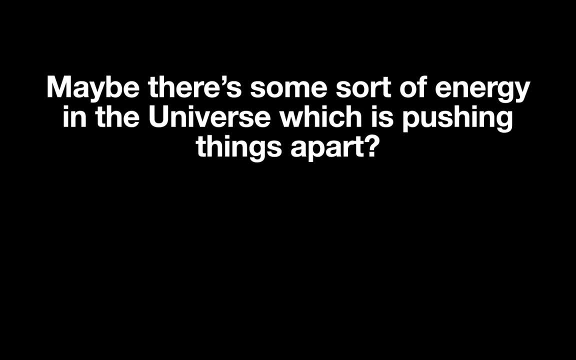 So it's an energy that we can't really notice on Earth because we're too small, But maybe just that there's a kind of energy in the universe that is just pushing things apart, And that's what we're seeing. An alternative idea is that maybe there's not energy in the universe. 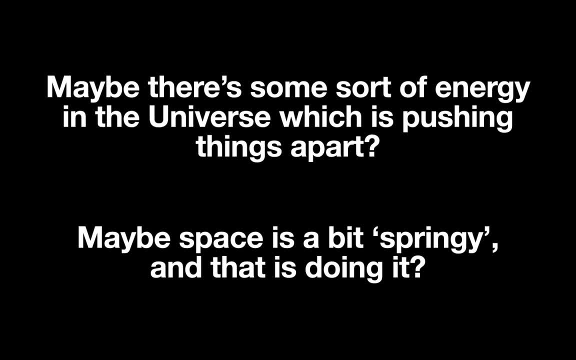 Any kind of stuff in the universe pushing it apart. Maybe it's space itself. that's a bit springy. If you imagine kind of squashing a spring between your hands, you would be able to feel it pushing back. Maybe that's what space does, right. 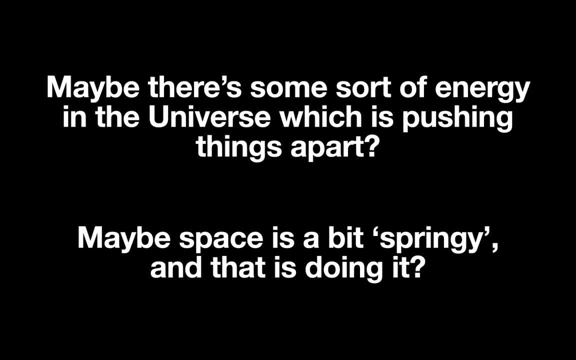 We know that space is bendy. That's what Einstein told us: that space is bendy. Maybe space is also a little bit springy and just kind of pushes back a bit when you push it back, And that's what's making the universe get bigger, faster and faster and faster. 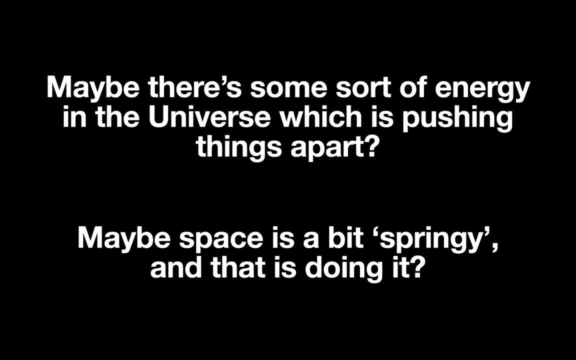 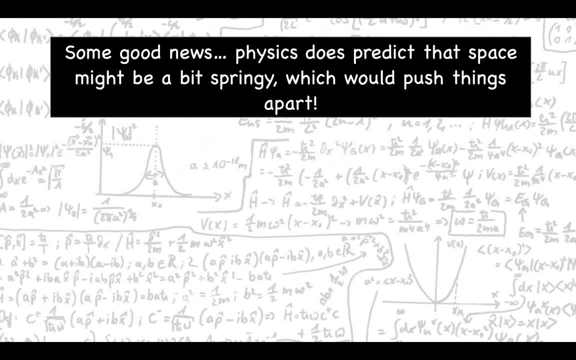 Maybe it's space itself just acting like a spring and kind of boinging the universe apart. There's something really interesting at this point. So if you go to your very, very complicated physics textbook, you will find out that physics does actually make a prediction that space is a little bit springy and would push things apart. 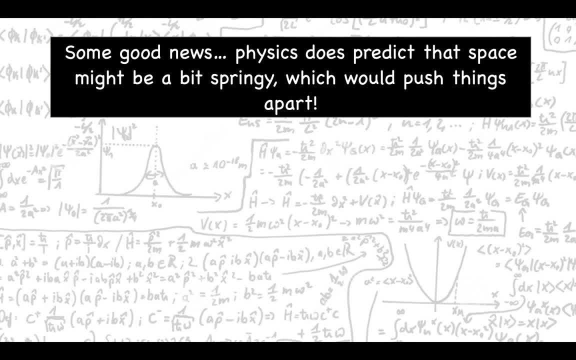 And you might think: well, that's fantastic news, We've solved the problem right. We see the universe getting pushed apart faster and faster and faster And there is a prediction from physics that space is a bit springy and will push things apart. 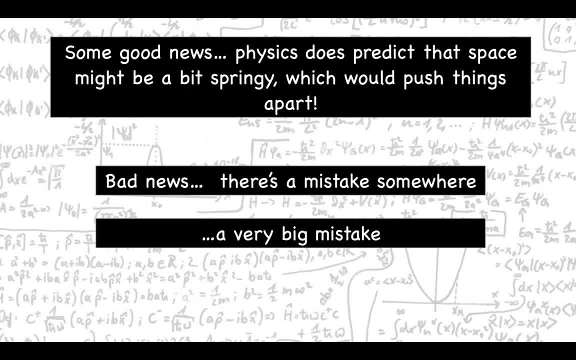 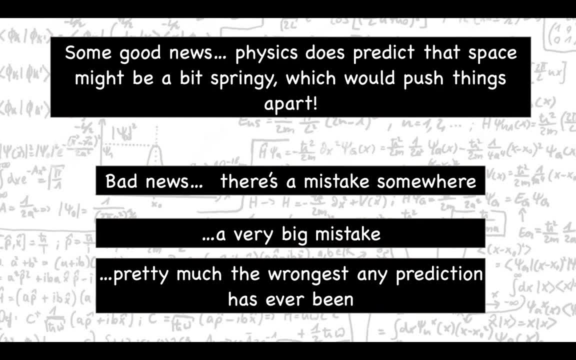 The problem. the bad news is there's a mistake somewhere- And it's actually a very, very big mistake, Which is that the complicated physics textbook kind of predicts how springy space is, but it's pretty much the wrongest any prediction has ever been, ever. 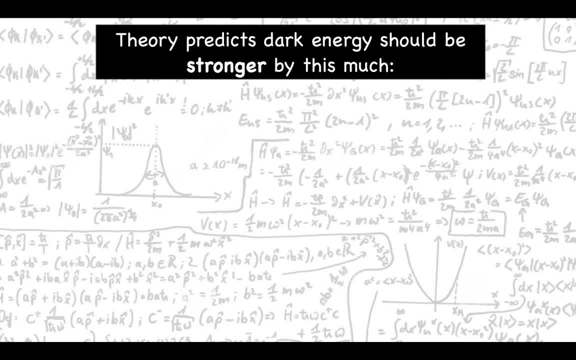 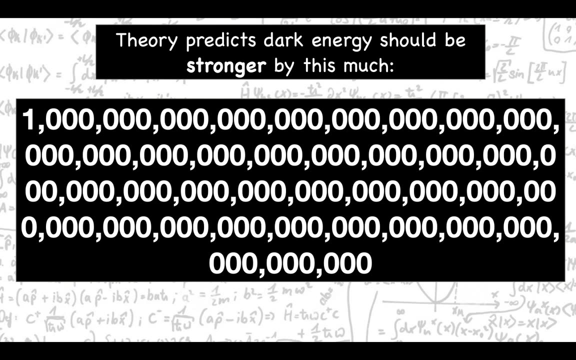 So the theory of the textbook, the physics book, predicts that dark energy, the springiness of space, should be stronger than what we actually see when we look around the real universe, And it predicts it is this many times stronger, Which is a very, very, very big mistake. 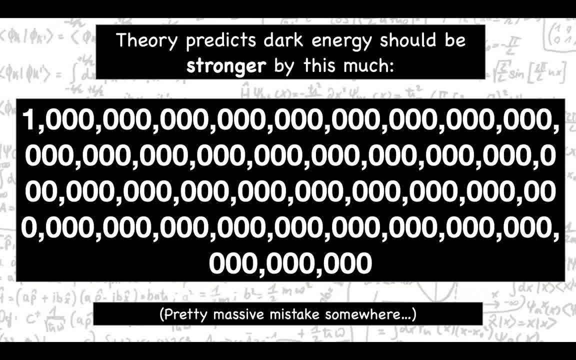 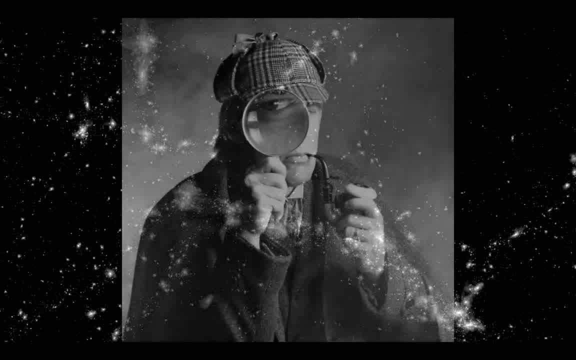 Very, very, very, very big number indeed. So you can see why I say this is pretty much the wrongest any prediction has ever been. So there's a very big mistake somewhere. So this is why I've said that dark energy is a real mystery, right? 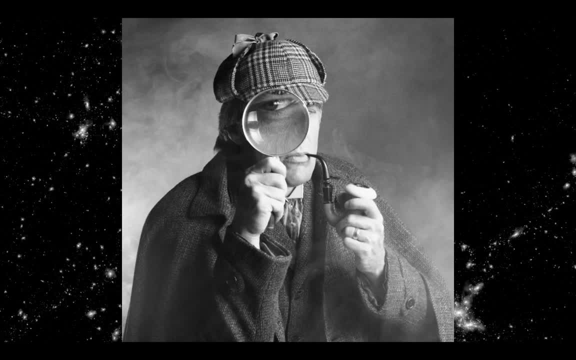 We really don't know what it is. It might be some thing in the universe that's pushing it apart. It might be the springiness of space. Right now we really don't understand. Dark energy is a mystery. We see it happening. 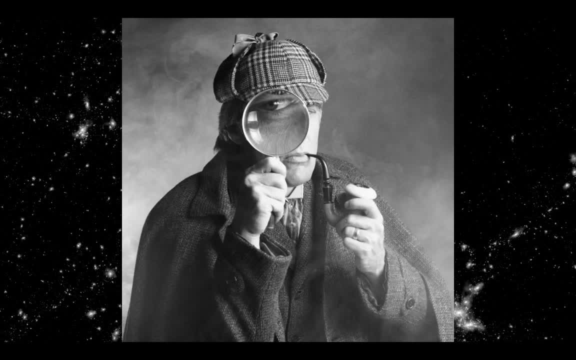 We see the universe getting pushed apart faster and faster and faster. We don't understand what it is at all, And so it's a detective story for the future. Right, So we have some of the clues, But what we need to do in the future is try and put these clues together and understand what's really going on. 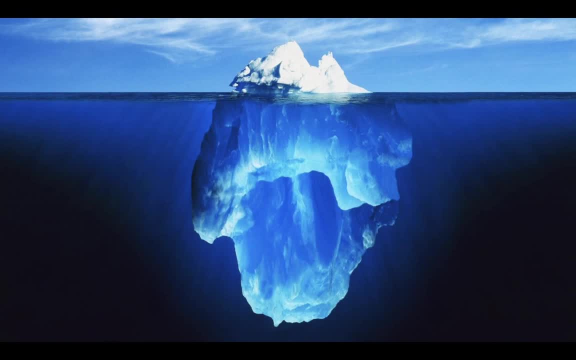 I'm going to leave you with one thought just before we go and do questions. Some of you might have seen pictures of icebergs before. Icebergs are really, really famous because only a little bit of the iceberg is above the water. 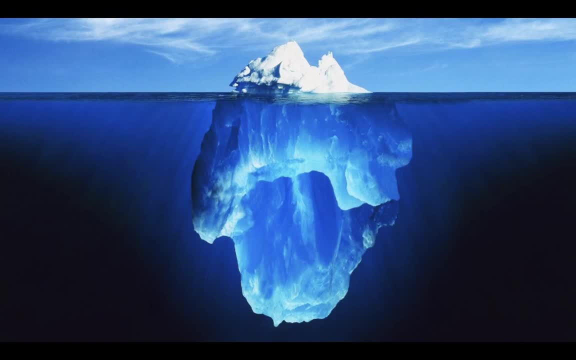 Almost all of the iceberg is kind of hidden and mysterious below the water, And this is kind of what our universe is like. So of our universe, something like five percent of our universe, is what we think of as normal stuff, And what I mean by normal stuff is the stuff that makes up, like me and you, and the earth and the sun and the solar system and all the stars in the sky. 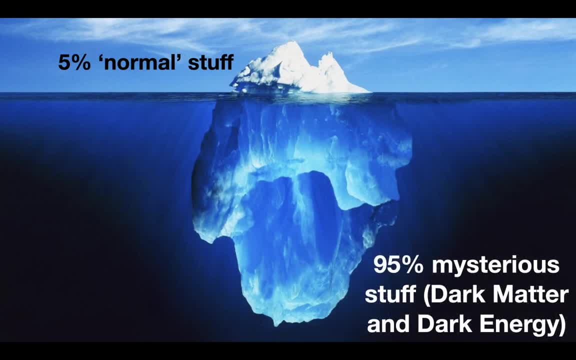 This is normal stuff, Dark matter and dark energy- the things that we've been talking about for the last couple of weeks- makes up ninety five percent of the universe, which is amazing to me, Right? So ninety five percent of the universe is almost all of the universe. 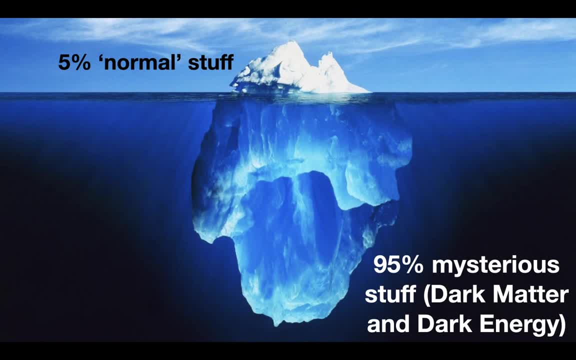 All the stuff that we're actually made of is almost an afterthought. Fully ninety five percent of the universe is stuff that we just don't understand very well, And some people might think this is quite a bad thing. I think this is a really 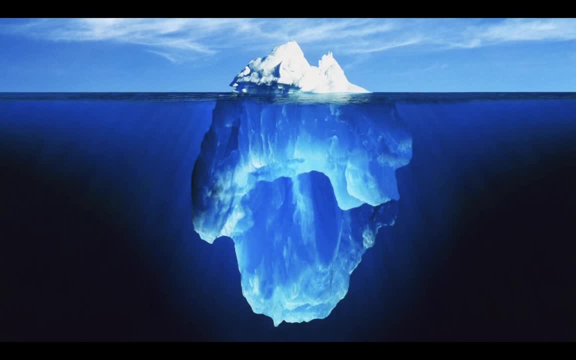 really good thing. as a scientist, I think this is really, really exciting because it means we just get to go and solve the problem. It's like being a detective faced with a really exciting mystery. We now get to go forward and try and learn what the universe is made of. 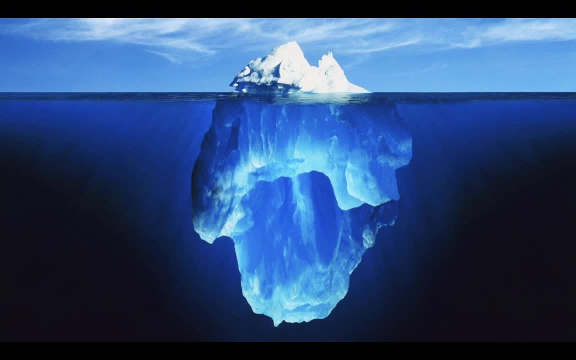 And so this is also a bit of a call for help, Right? So we are looking for young people who find this topic really interesting To study hard and become scientists and help us solve this problem, because we're going to need people to help us solve this problem in the future. 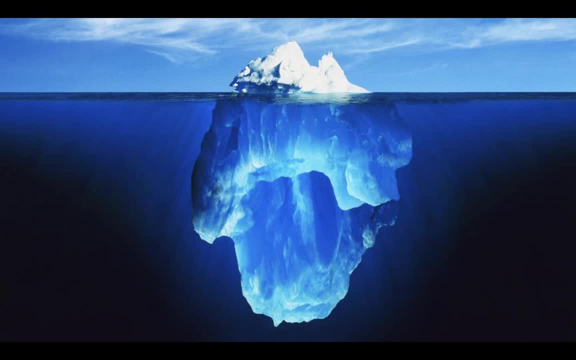 It's one of the most exciting problems the human race has ever faced with, Right, What is almost all of the universe made of? And I can't wait to find the answer. Okay, We've been going for nearly half an hour. I think that's a perfect time to finish. 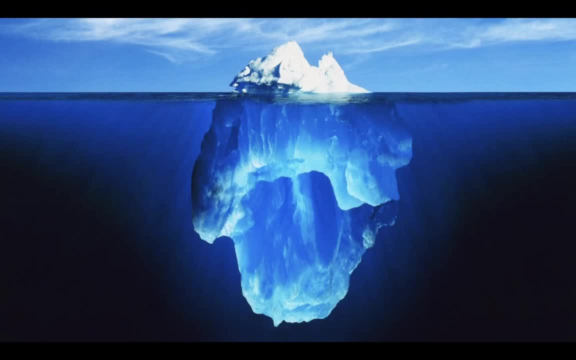 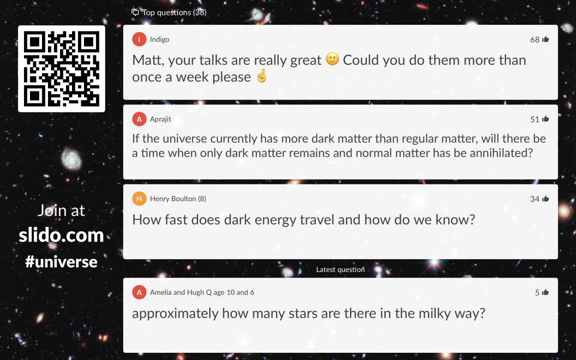 What I want to do now is go over and answer some of your questions. Let's have a look Um top question. I would love to do one of these. Uh, I would love to do these talks more than once a week. 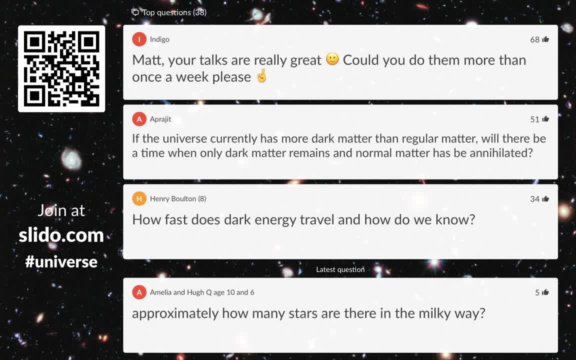 Um, I I wish I could uh writing. these is quite a lot of work and I don't think I have time to make more than one a week. I'm very sorry, but I will carry on doing them um as long as I can. 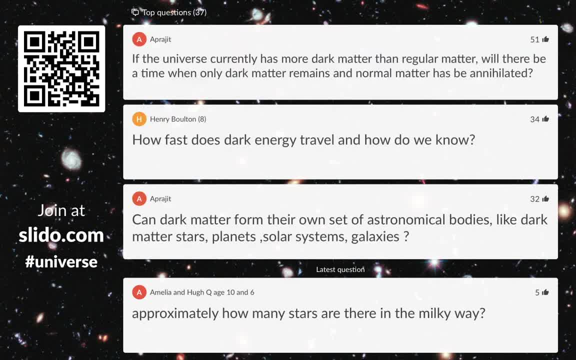 That's very kind of you. Um, a project asks: uh, if, if the universe currently has more dark matter than regular matter, will there be a time when there's only dark matter left? And the answer is yes. So this is a very, very long time in the future, right? 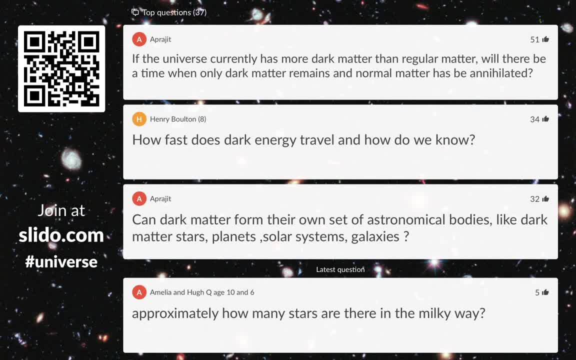 So once, Uh, all the stars have died out- This is kind of countless billions of years- in the future, There will only be dark matter left. That's right? Um, so if the big freeze is the right answer and the universe just gets bigger and bigger and bigger forever in the way, way, way, way, way distant future, the universe will just have dark matter in it. 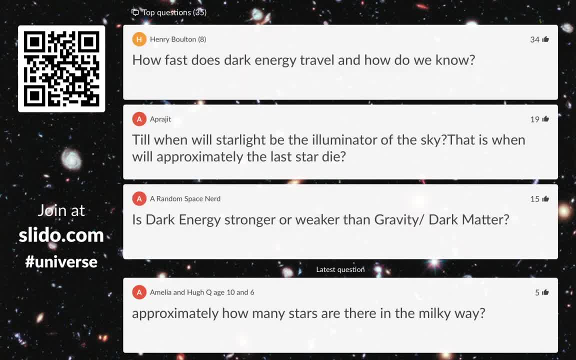 So the answer is yes. Uh, Henry Bolton says: how fast does dark energy travel and how do we know? Um, so the the the answer to almost all dark energy questions has to be: we don't really know. dark energy is a real mystery, right. 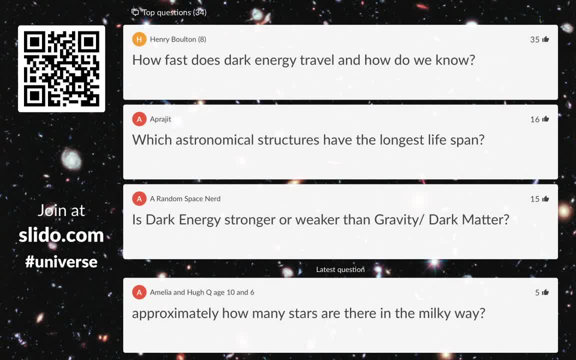 Our best guess is that it's not a thing that travels from space like from place to place. It's probably a thing that kind of fills the universe, So a bit like being a fish kind of inside the sea. right, The sea would be just absolutely everywhere. 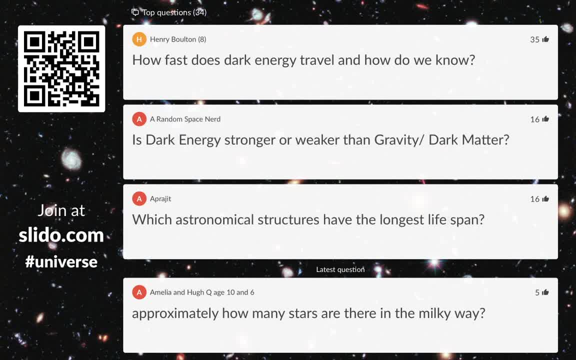 It'd be. the sea would be above you and below you, and in front of you and behind you. That's probably what dark energy is like in our universe, right, It's probably a thing that is just absolutely everywhere It's. It's not a thing that travels from place to place and uh, but, yes, but remember that with most, most things in the universe, um, uh sorry, with most things to do with dark energy, uh, everything is a bit mysterious because we don't really understand dark energy very well at all. 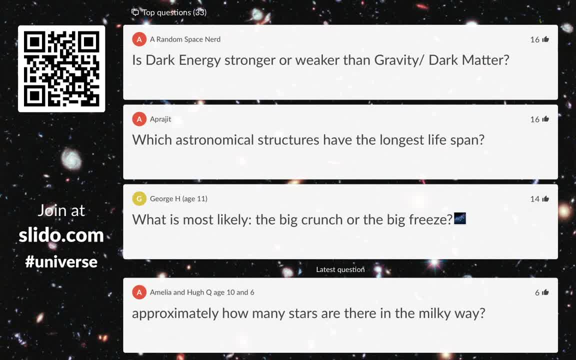 Um, a random space nerd says: is dark energy stronger or weaker than gravity and dark matter? Um, it's very, very hard, So we're slightly comparing apples and oranges here. It was quite hard to say, Um that, whether things are stronger or weaker, I think the best way to describe it is that dark, uh, dark matter and gravity win on small scales, but dark energy wins on big scales. 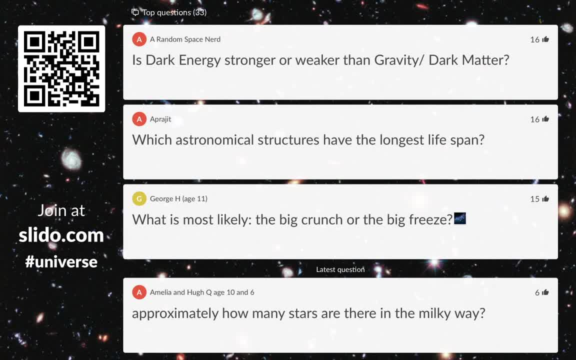 And so you know, we, we obviously gravity wins on small scales, right, Because if you, if you throw a ball up in the air, dark energy doesn't make it whoosh, apart from the earth. right, On small scales, like, um, like people scales, gravity wins. 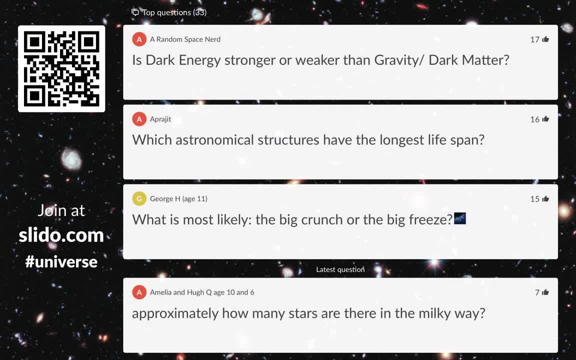 And- and that's that's even true If you think about our solar system, right? Uh, the earth is orbiting around The sun. because of the sun's gravity, dark energy isn't pulling the earth and the sun apart, right? 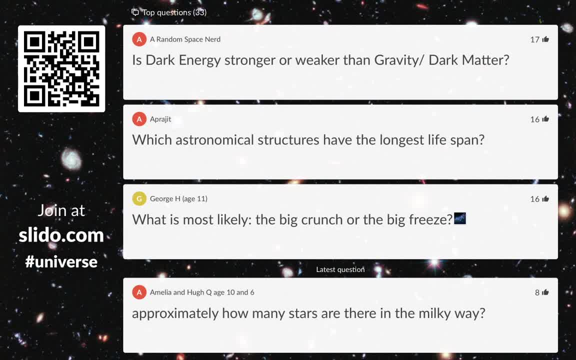 We're staying the same distance apart, because gravity is stronger, and the same is even true on the scale of our galaxy, right? So from dark energy's point of view, even the galaxy is quite small, So our Milky way galaxy is not getting bigger, right? 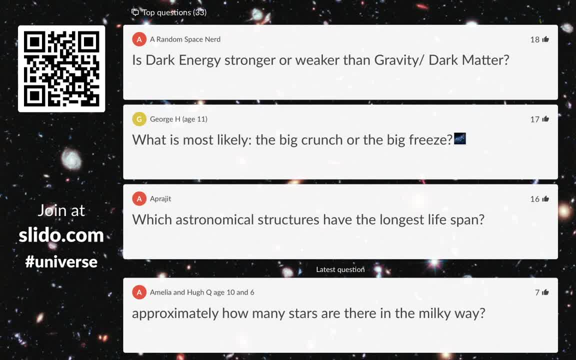 Our Milky way galaxy is being held together by gravity, Um, but over very, very, very, very long distances, so millions and millions and millions of light years. dark energy is stronger, And that's mainly because gravity gets weaker the further you go away, right? 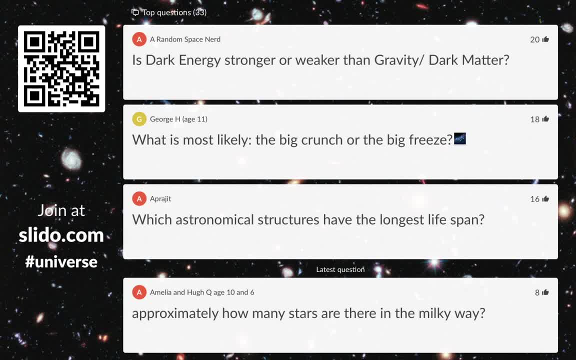 When he travels away from something, the gravity of it gets weaker and weaker and weaker. But as you travel further and further away, dark energy just seems to get stronger and stronger, And so that's why, over millions and millions of light years, dark energy wins. 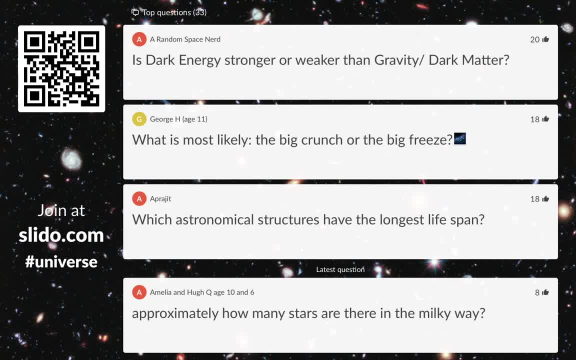 So for small things- and by by small I mean like galaxy size or smaller gravity wins. For really big things, dark energy wins. Um, but there we go. Take this one off. Uh, Abrogit asks Which astronomical structures have the longest lifespan. 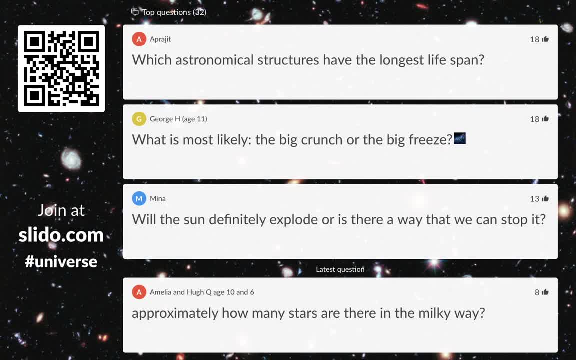 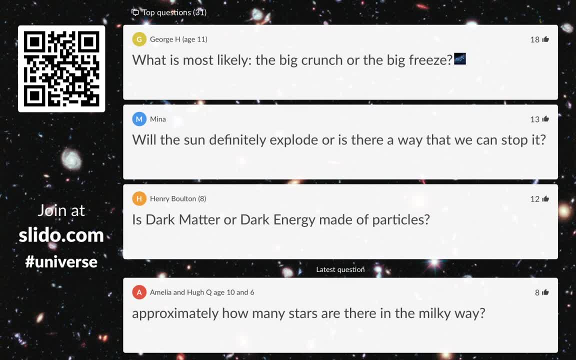 Uh, so the thing in the universe that will live the longest are black holes, by a very, very long way. Uh, so the far, far future of our universe, uh, once all the stars have died out, will be a universe just full of black holes. 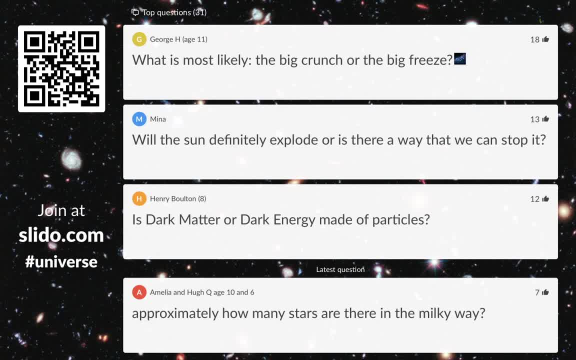 The last things in the universe to vanish will be the supermassive black holes in the middle of galaxies. Uh, so black holes are the longest lived by a very, very long way. Uh, George H, age 11, asks What's the most likely. 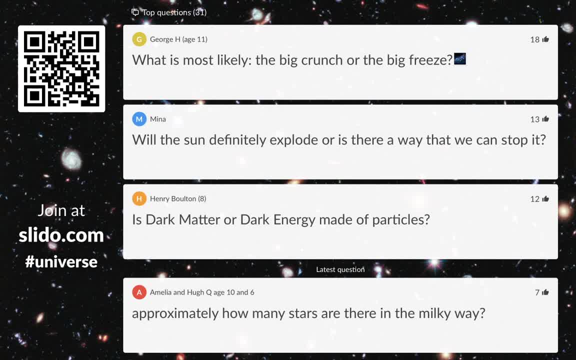 The big Crunch or the big freeze. Um, I'm hoping we answered this one. Um, we think that's because we see the universe is getting bigger and bigger and it's getting pushed faster and faster and faster. apart, The big crunch is probably not going to happen. 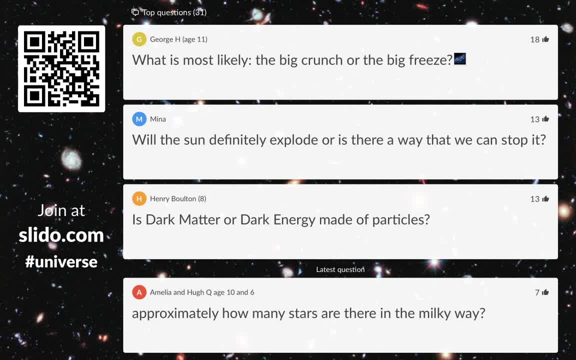 And so, uh, the big freeze is the most likely one, which is good news. Um, Mina, asking another question about the future of our universe: Will the sun definitely explode, or is there a way we can stop it? Um, so, the sun. 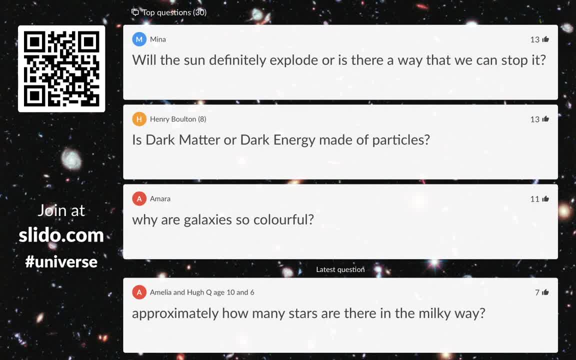 Is going to die. Unfortunately, it's going to take a very, very long time. It's going to take something around four or 5,000 million years in the future. There's probably no way we can stop it, though, because the sun is burning all the time. 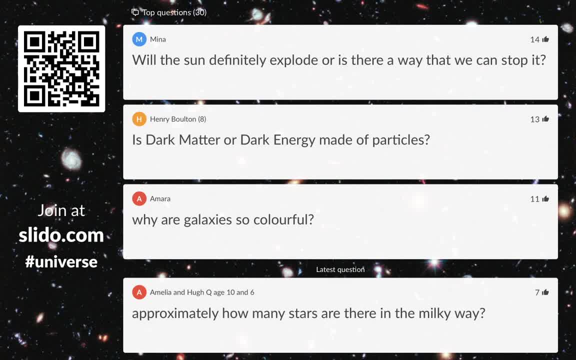 And all the while the sun is burning, it's using up fuel, right Like a car driving down the motorway using up its petrol, And we can't stop it from using up its fuel because you know, then then some would go out. 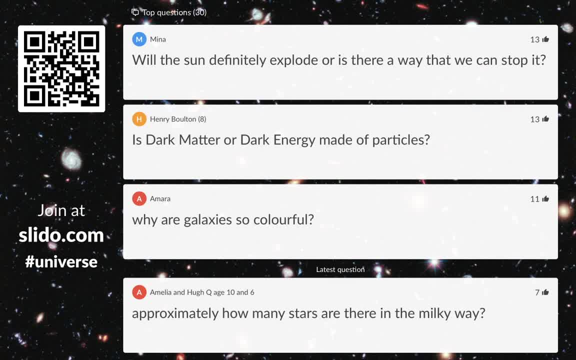 That's not what we want, right? We want the sun to carry on burning because it keeps us alive, and one day it is going to run out of fuel and die. Um, but Luckily it's going to. not, it's not going to happen for thousands of millions of years. 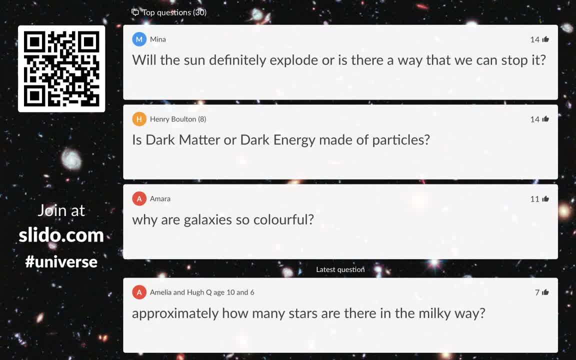 And in that time that gives us enough time to find somewhere else to live. Hopefully we know about lots of other planets in the universe that are habitable, that are nice for life, And so there's not much we can do to stop it. 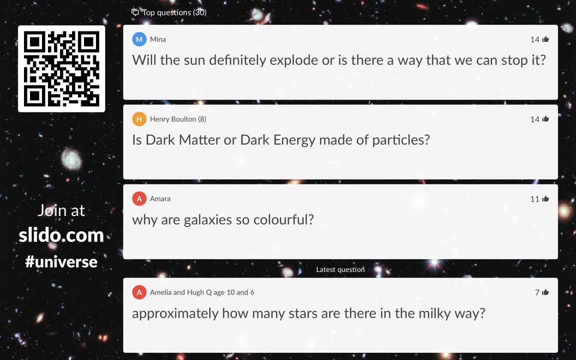 But what we can do is find a new home, uh, where uh we can. we can carry on living even when the sun has died, But happily we have thousands, of millions of years to work something out. Uh, Henry Bolton, age eight, is asking some fantastic questions. 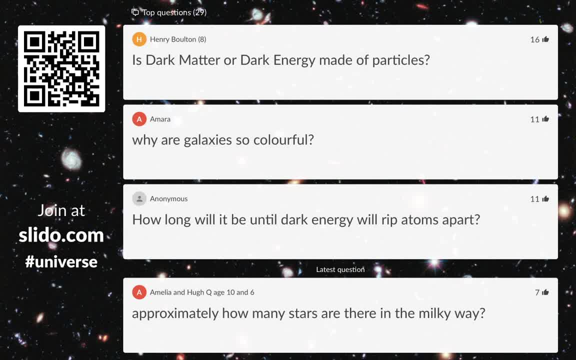 Henry, is dark matter or dark energy made of particles? Um, again, this has to be. uh, this is what we prob. this is what is probably the right answer. Um, dark dark matter and dark energy are both really, really mysterious. 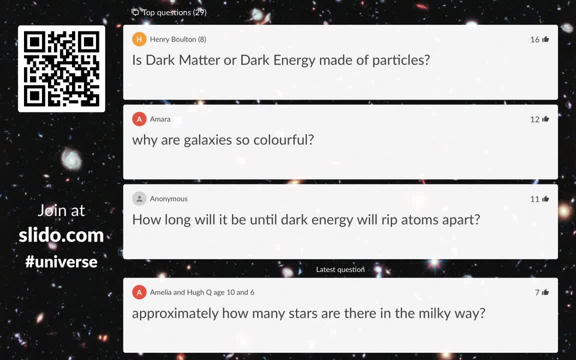 But our best guess is that dark matter is made of particles and dark energy is not made of particles. So we think that dark matter, of these lots and lots of tiny, tiny particles that fill up the universe, dark energy is probably some kind of like energy thing that's pushing the universe apart. 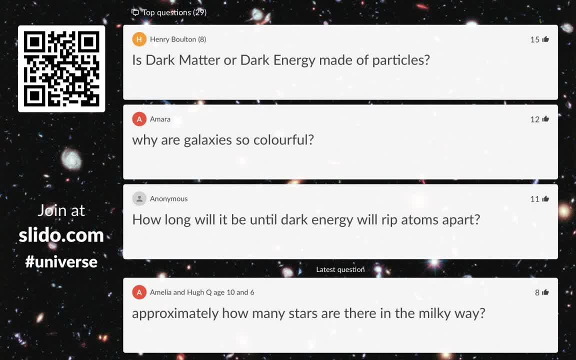 Um, so, yeah, dark matter, yes, dark energy. no, very good question, Henry. Um, if you, if you didn't see the dark matter talk last week, check that one out. That's going to tell you all about why we think, uh, dark matter exists and what we think it does. 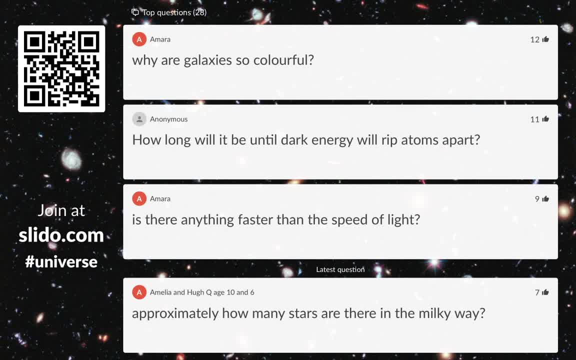 Amara is asking a fantastic question: Why are galaxies so colorful? Uh, you're right. So I showed you these pictures of galaxies, uh, before, if you remember. and they are. they are very, very colorful indeed. Galaxies are colorful because they have lots of different things in them. 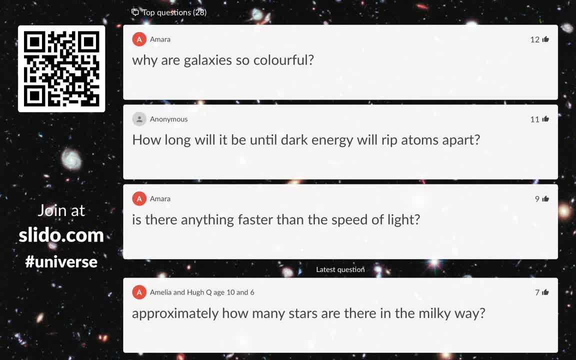 Uh, so So partly is: galaxies are made of stars, and stars are all different colors. We have blue stars and we have red stars and we have orange stars, And so the color of galaxies come from their stars A lot of the time. galaxies also have lots of dust in as well. 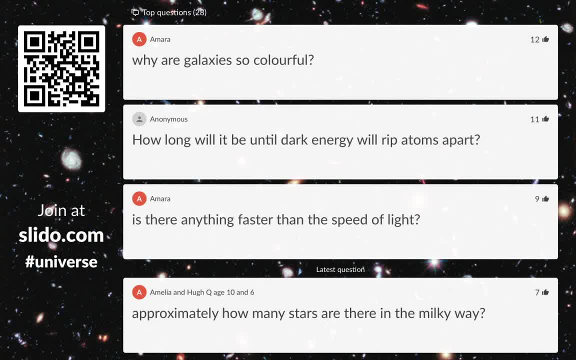 And dust can kind of glow with exciting colors when, uh when, stars are inside them. Um, so galaxies are so colorful because the things that make up galaxies, like gas and dust and stars, are themselves really, really colorful. Um, it's a good question. 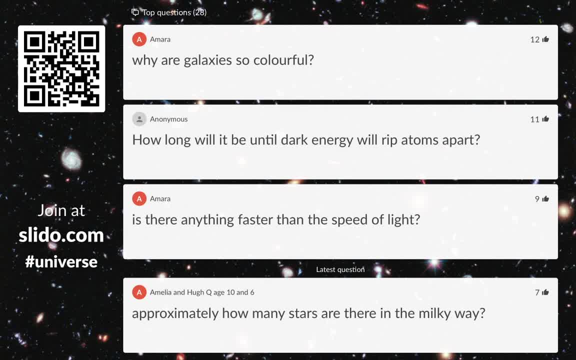 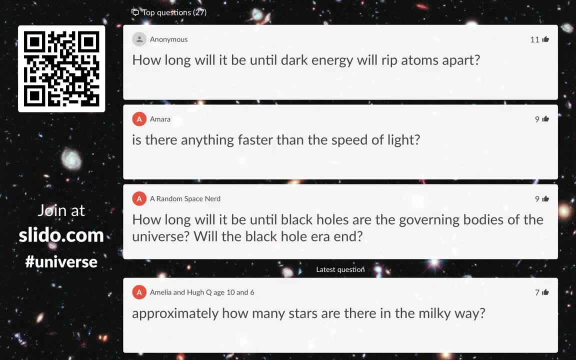 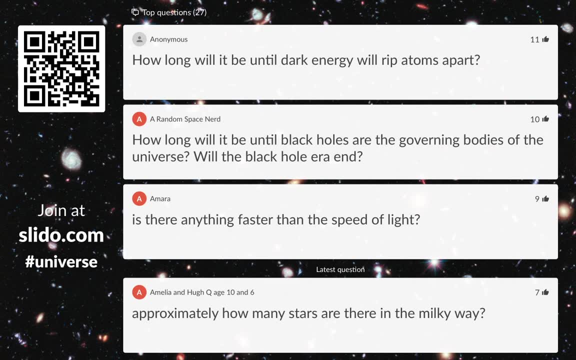 I, I absolutely love pictures of galaxies. Uh, galaxy pictures are can be very, very colorful and amazing. Um anonymous asks: how long will it be until dark energy rips atoms apart? Um, so the first thing I have to say, like I'm saying over and over again, we don't totally know, right? 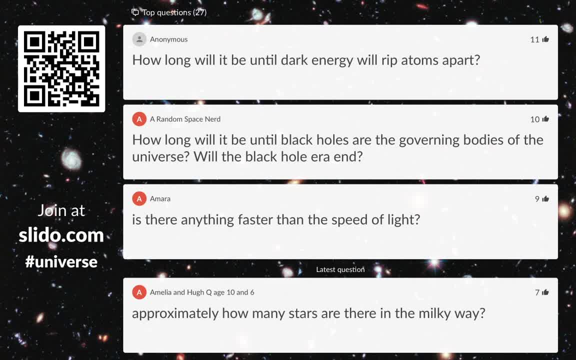 The big rip might or might not happen. There are some theories that say the big rips going to happen. There are some theories to say it won't. Um, the best guess that I've heard, for if the big rip is going to happen, it's going to happen in something like 20 billion years. 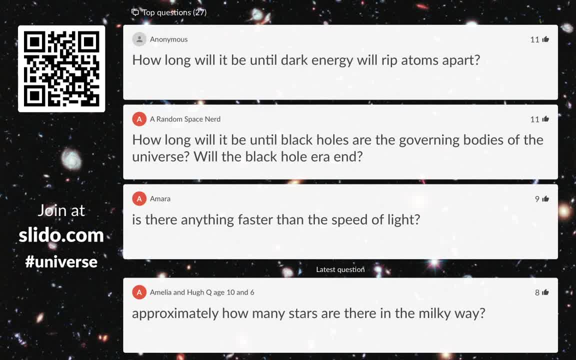 Time. So a long, long, long, long time after, uh, the sun uh has gone out. um, this is, if it happens at all, Right, But the best uh some of the guests I've heard, or some of the theories I've heard, uh, for the big rip is in about 20 billion years time. 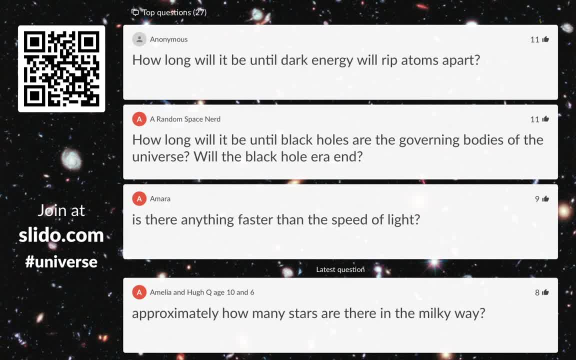 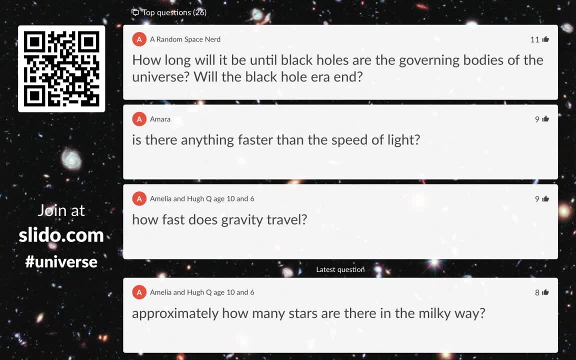 So that's a pretty good, reasonable, uh estimate. Um, a random space nerd says how long will it be until black holes are the governing bodies of the universe and will the black hole era end? So right now we are In, uh, what sometimes gets called the stelliferous era, which I absolutely love that word. 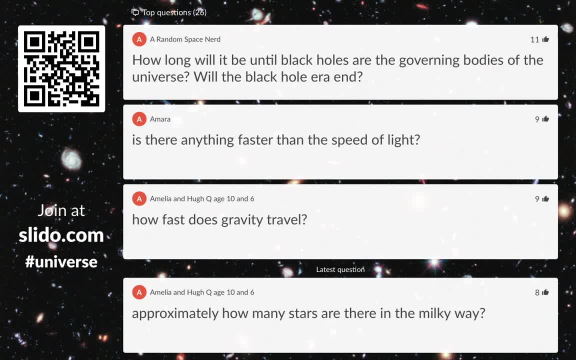 Stelliferous- Um, it's basically a fancy word meaning full of stars. Uh, so our universe is full of stars right now. right, When we look around the universe, we see loads of stars. Stars are the main things that are dominating our universe right now. 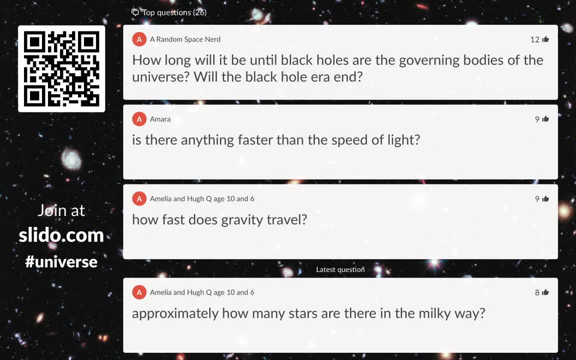 But as time goes by, just like the sun is going to end- that we've been talking about already- Um, eventually all the stars are going to end, right? All the fuel for all the stars in the universe is going to run out. 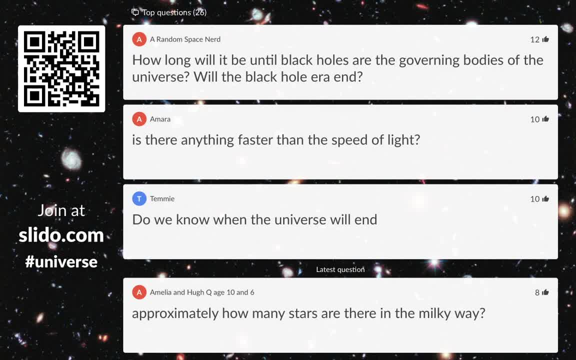 And at that point the black holes will be Left. this is going to happen a very long time in the future. Um so, big stars die very quickly, but small stars take a very, very long time to die. Like a very, very small red dwarf star, might live for a hundred billion years or more. 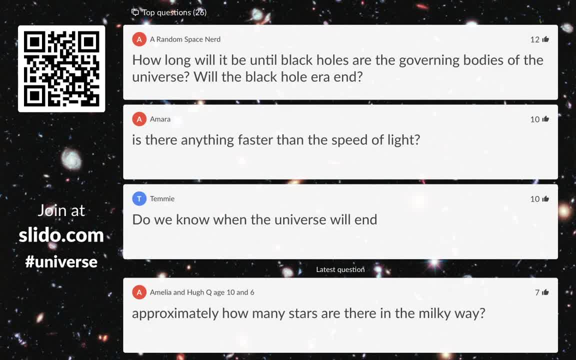 Um and so, and of course, some of these red dwarf stars haven't even been born yet. Um so, given that the big rips not going to happen, we'll assume that we living in a big freeze universe that's going to get bigger and bigger forever. 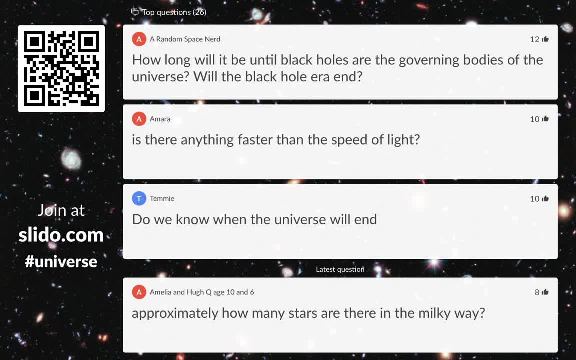 It might be something like a trillion years. It might be Like it might be. it might be a thousand billion years, until the last stars die, And at that point, uh, there'll be just black holes left. The black hole era will end as well, because even black holes die eventually. 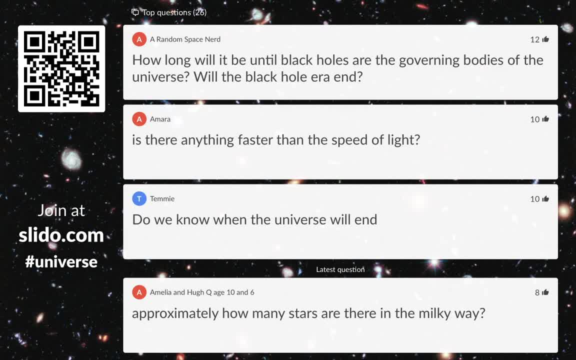 This is why one of Stephen Hawking's most famous results- that black holes actually evaporates. It happens very, very, very slowly, So the black hole era will indeed end, but it will happen in an amount of time that even makes a trillion years look like a second. 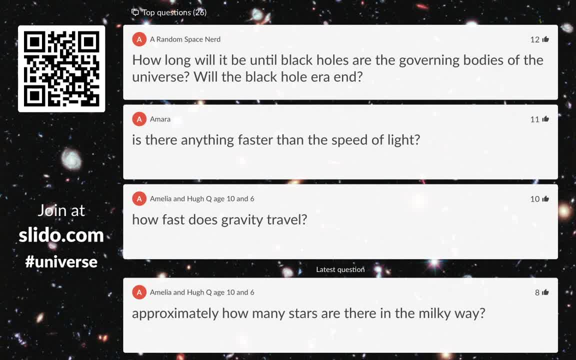 It will be an unbelievably long time Until the black hole era ends, at which point the universe will be kind of full of nothing. We're still just getting bigger and bigger and bigger forever. Uh so, uh yeah. so black holes will kind of take over in maybe, maybe a trillion years. 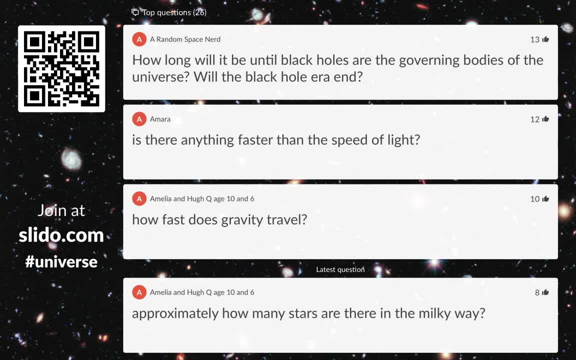 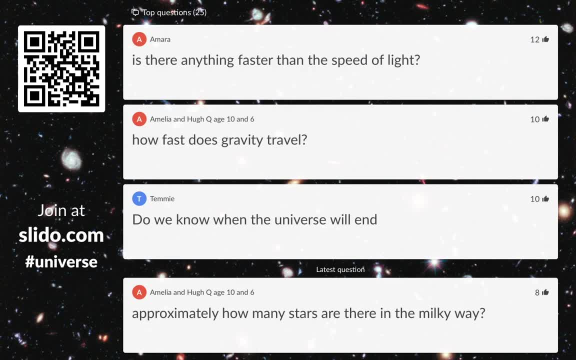 Uh, will the black hole era ends? The answer is yes, but in such a long time. there's not even a word for it. Um Amara says: is there anything faster than the speed of light? Um, so generally, the answer is no right. 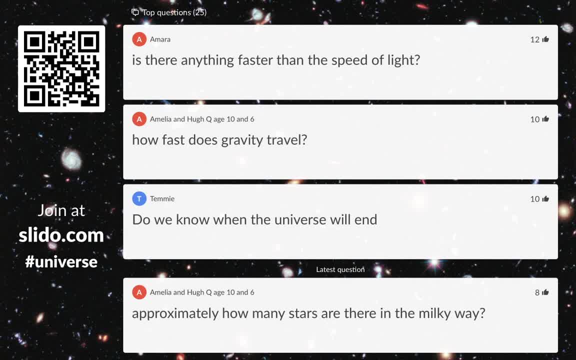 So nothing can travel faster than the speed of light. Um, if you kind of throw a ball, the fastest it could possibly go is the speed of light. and an interesting answer to this, which gets a tiny bit complicated, is that the expansion of the universe can actually go faster than the speed of light, because we're talking about the universe getting bigger and bigger and bigger, and that can actually happen faster than the speed of light. 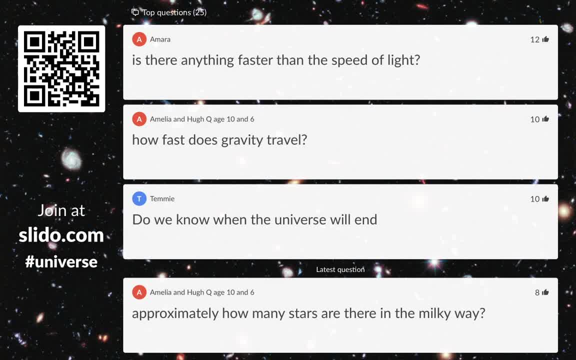 There can be a galaxy on the other side of the universe that's moving away from us faster than the speed of light, and that sounds kind of bonkers, right, Because we we just said the rule is that nothing can go faster than light. 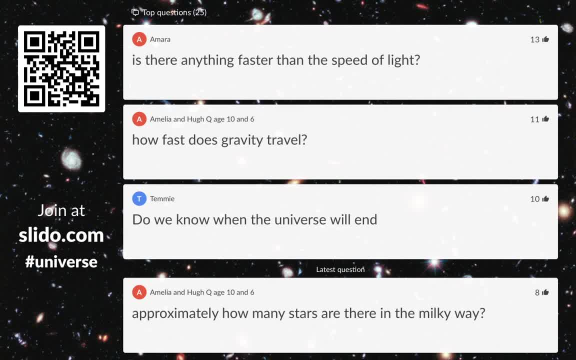 How can the universe Expand faster than light? The answer is that the, the, the the speed limit of the speed of light, saying the speed of light is the fastest thing there is. That refers to kind of objects moving through the universe, right? 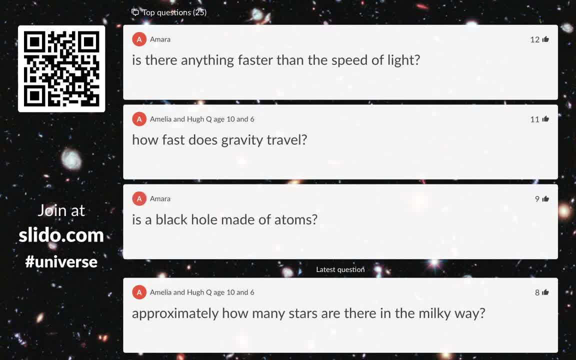 Like if you're a car driving down the motorway, you'll see you're an object moving through space- right, And the speed of light is the fastest you can go. but distant galaxies aren't moving away from us, because they're moving through space. 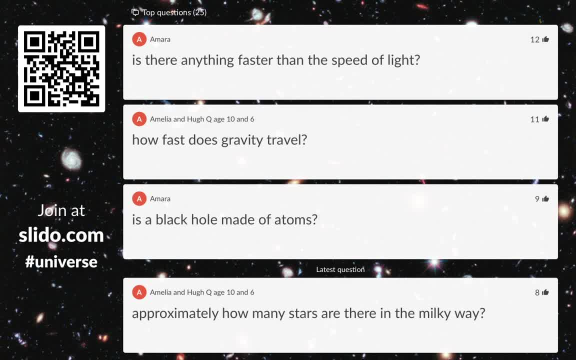 It's actually space itself getting bigger and bigger and bigger. The universe expanding. Isn't things Moving through space? is the whole universe blowing up by a balloon And, as far as we know, there are no rules to say how fast that can go. 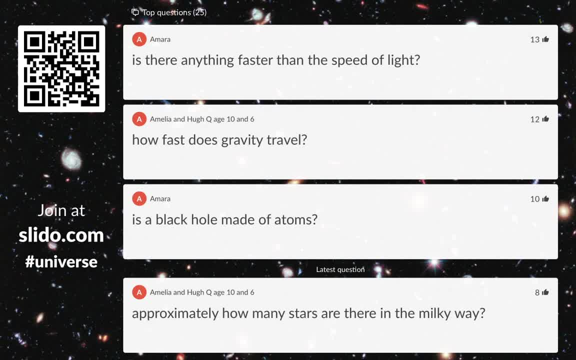 And so, in terms of actual things moving around in the universe, the speed of light is the faster that can go, but the universe itself, um, can go faster. Amelia and Hugh Q, age 10 and six, ask a very excellent question, which is: how fast does gravity travel? 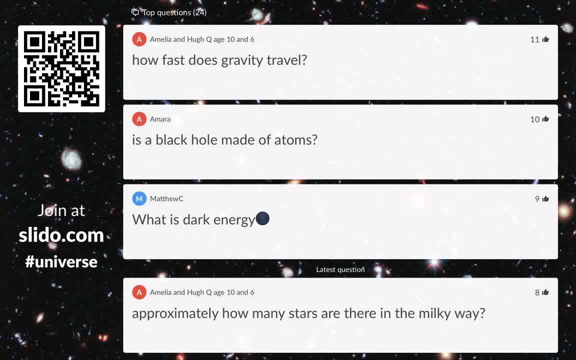 And this comes into the question that just got answered last time. Uh, the answer is this: The speed of light. uh, the speed of light is the fastest that anything can travel around inside the universe, and gravity travels at the speed of light, which is kind of fascinating. 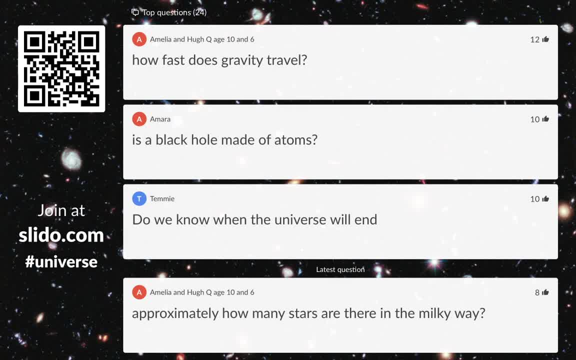 If you think, um, if you had a magic wand and you could make the sun disappear, that means that earth would carry on orbiting for about eight minutes, Cause that how fast the speed of light takes between the sun and the earth. So we would carry on orbiting for eight minutes until, like, the signal reached us and we kind of flew off into space. 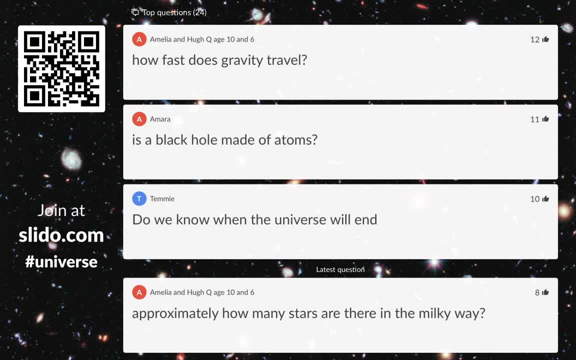 Um, so yeah, gravity travels at the speed Of light. Amara, asking some fantastic questions: is a black hole made of atoms? Um, they're made of atoms originally, right? So again, if you go back a couple of weeks, so we have a talk on this channel all about black holes. 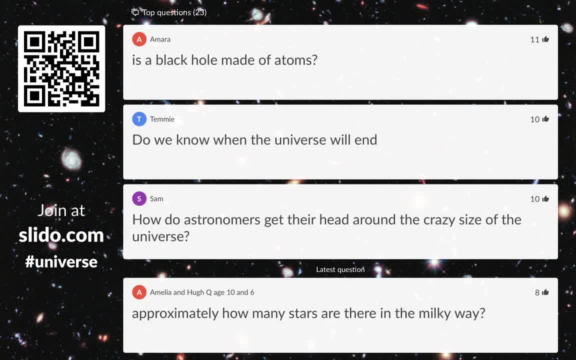 And I explained that one of the main ways black holes die. is that also one of the main ways black holes form? or when big stars die, right? So you take a star, you squish it up small and you make a black hole. The star that forms a black hole is made of atoms, right? 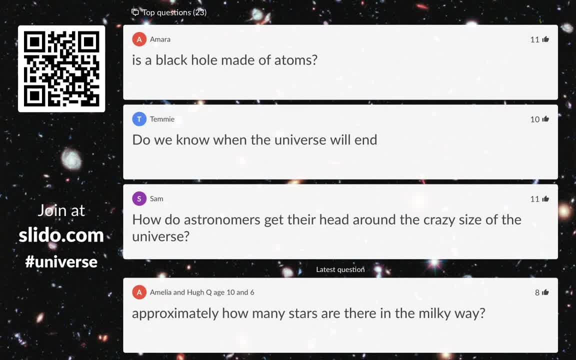 So atoms are the stuff that you make a black hole. It's made out of originally. um, but a black hole. what is the? the actual thing that forms a black hole is when you squish things up until they're just, until they're nothing, that's until the atoms don't even exist anymore. 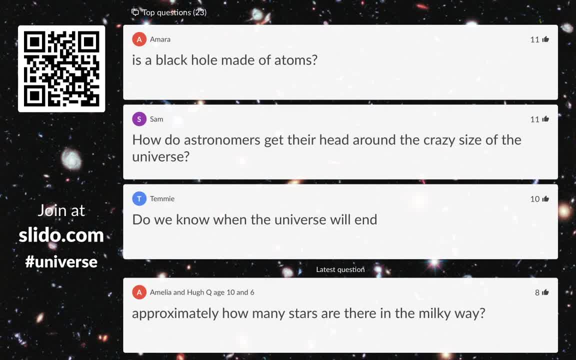 So a black hole is what the some atoms are, what a black hole is made of originally. but the actual black hole itself, um, is not made of atoms. It's made of something very, very strange called a singularity, which is a tiny spec, much smaller than an atom that weighs as much as a star. 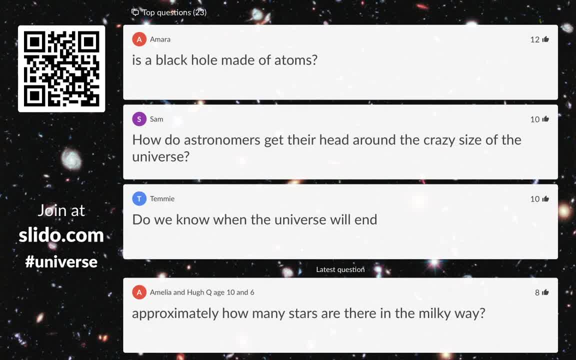 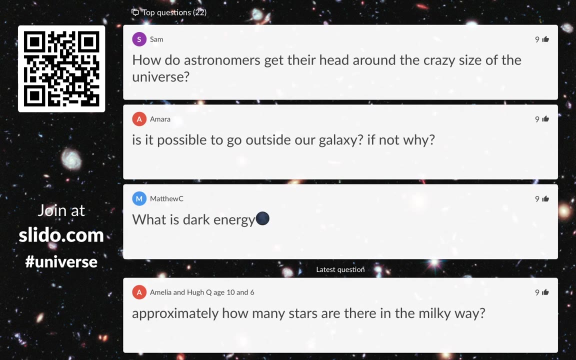 So atoms are what goes in, but an atoms Aren't What A black, A black hole, actually is? um, Sam asks: how do astronomers get their heads around the crazy size of the universe? I really love this question. Um, in a way the. the answer kind of is: you don't? um, astronomers are very you know. we go around saying so many millions of light years away and these things. um, you kind of just have to accept that you can't, that it's too much for your brain to understand. 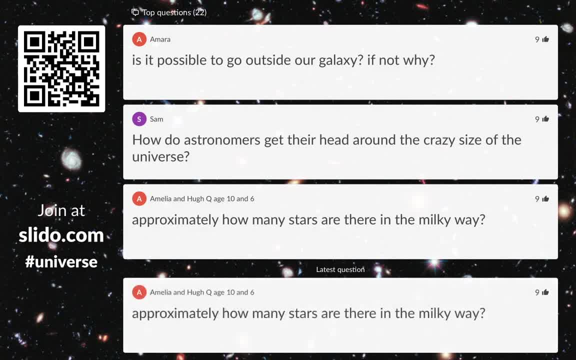 Right, Um cause, if you think about it, like our, our minds, our brains, Like didn't evolve to be able to understand the size of the universe, Right, We, under our minds, evolved, our brains evolved to understand the stuff around us like things that are millions and millions and millions of light years away. 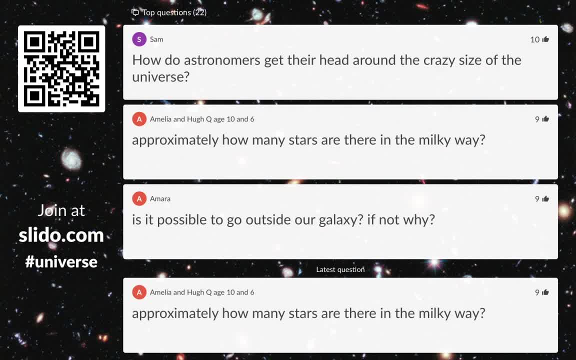 I just um, it's just, yeah, it's beyond anything that we evolved to understand, And so I think part of being an astronomer it's just accepting that you're not going to like truly understand it. Uh, that doesn't mean we don't understand it from like a like a kind of math point of view. 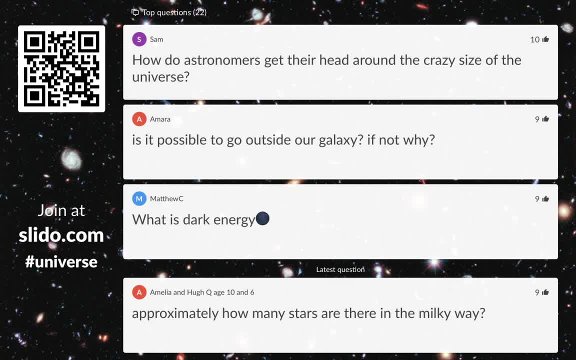 Right, Like we can, kind of like we can do the sums on the paper and, like you know, we can take Measurements from our telescopes and it all makes sense. but as far as I actually kind of deep down understanding in your head what millions of light years really, really means, 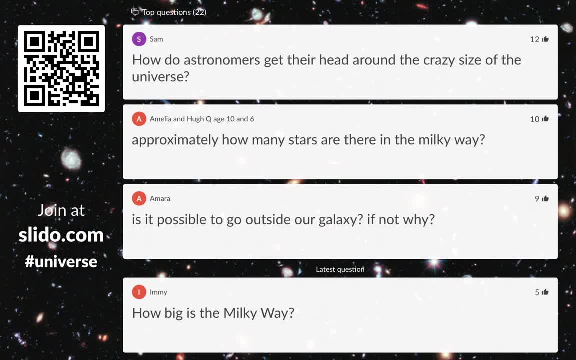 Um, I think you just have to accept that you can't. uh, people are far too tiny to really understand, uh, this crazy size of the universe. That's a fantastic question, Sam. Well done, Amelia. and Hugh again asks how many stars are there in the Milky way? 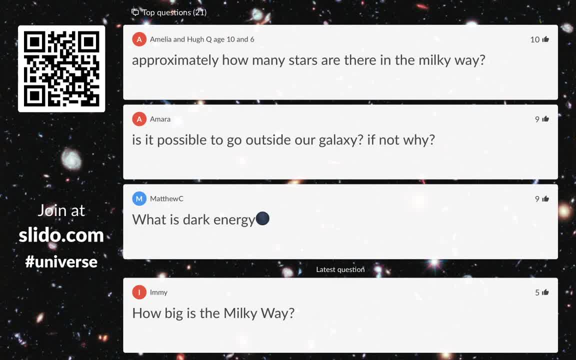 Um, we don't know for sure, Something, uh, somewhere around somewhere between 200,000 billion and 400,000.. So Look, Yeah, Yeah, Yeah, Yeah, Yeah, Yeah, Yeah. So, um, it's a 200,000 million to 400,000 million. is that kind of the the range of? 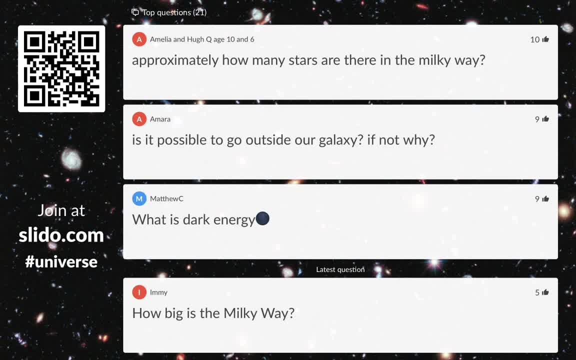 estimates, So between about 200 billion and 400 billion are the best answers. Um. Amara, asking another really good question: Is it possible to go outside of our galaxy? Um, there's nothing stopping us, apart from how far it is. 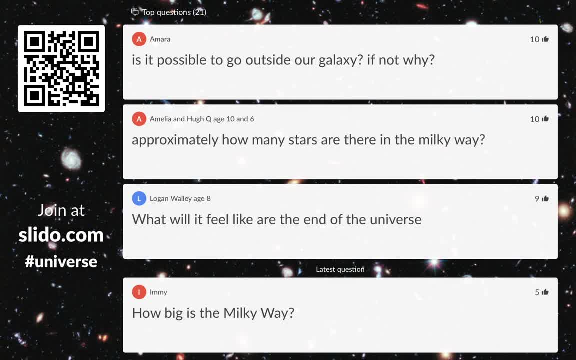 Um, so if you think about the nearest star to us, it's called Proxima Centauri. the fastest thing humans have ever built would take, uh, take- hundreds of millions of light years, of thousands of years to reach, and that's even the nearest stars. um the fastest rocket we've 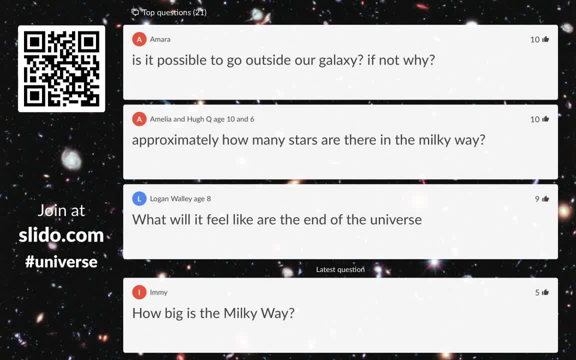 ever built would take billions and billions and billions of years to leave our galaxy. so the only thing that's stopping us is just how very big our galaxy is, and i've already answered that one. uh, logan wally aj said: what will it feel like at the end of the? 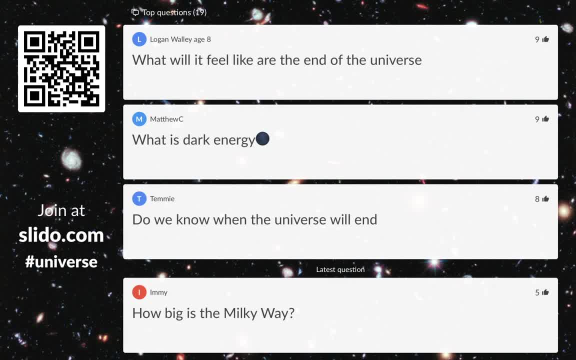 universe. um, this is a great question. well, it kind of it depends what the what. the end of the universe is right. if the end of the universe is a big freeze, uh, then it will just be a big empty universe with nothing in it at all, because the big freeze goes on forever, right? so that means the last stars. 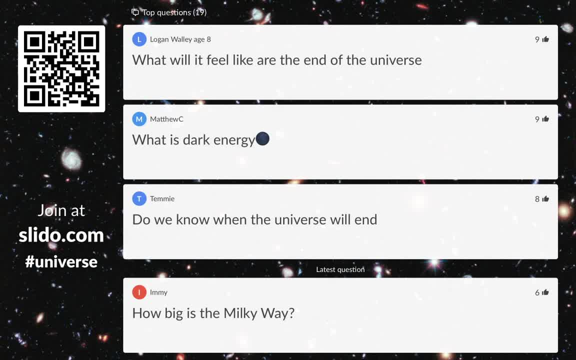 die, the last black holes evaporate and you just end up with a universe that's just full of nothingness, just getting bigger and bigger and bigger forever. so if that's what the end of the universe is, then it will just be very, very cold and very, very dark forever. um, if the big rip happens, 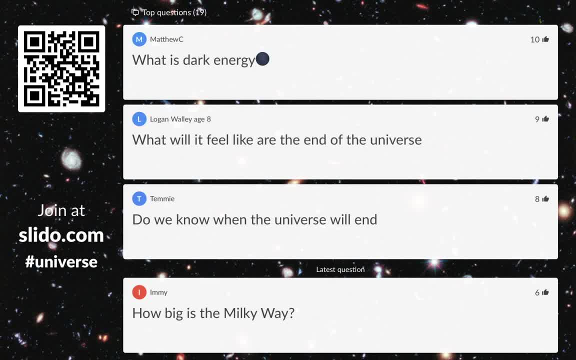 or the big crunch happens, it's likely to be a lot more exciting, but it's very, very hard to imagine, so we don't totally know what the answer is. what the answer is depends on what the end of the universe is going to be. matthew c says: what is dark energy? i would love to give you an answer. 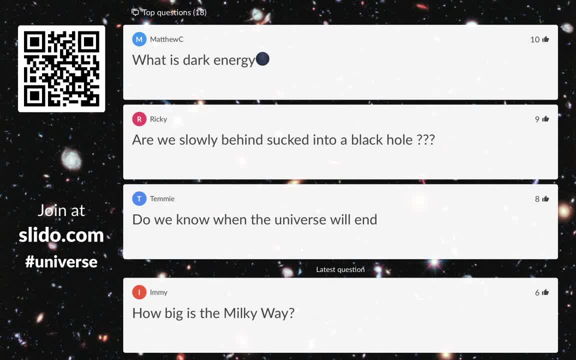 to this: uh, the answer is, right now that no one really knows. uh, maybe, uh, maybe we need one of the people submitting questions today to become a scientist and uh and solve the question. uh, right now we don't know. it's one of the biggest mysteries. um, i'll do a few more for a few more minutes. 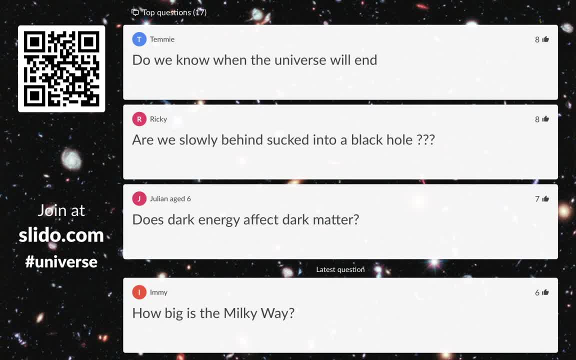 um temi says: do we know when the universe will end? um again, it depends on what kind of end the universe has, right? so if the big rip is how the universe is going to end, like that, that's, the universe being torn to pieces by dark energy- then that will happen in maybe 20 or 25 000 million. 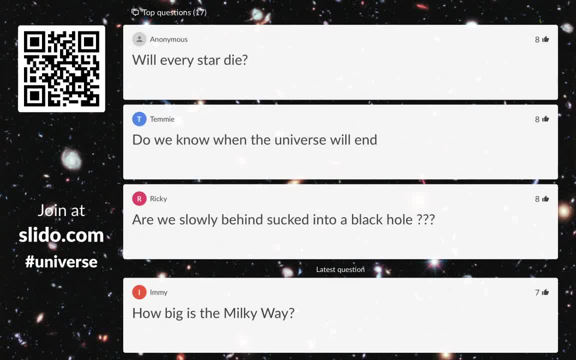 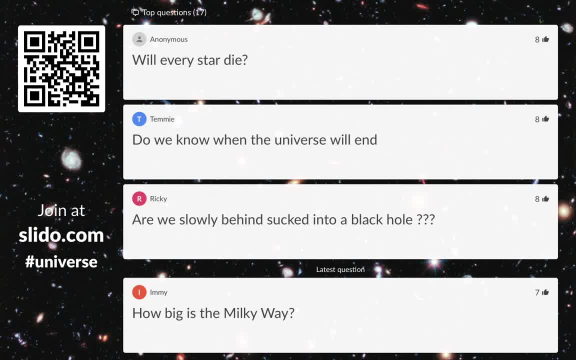 and bigger forever, and that's that just goes on until the end of time. um, so yeah, that one again depends on what the actual end of the universe really is. okay, i think i'll make this the last question, because we've been going nearly 50 minutes. the anonymous says: will every star die? 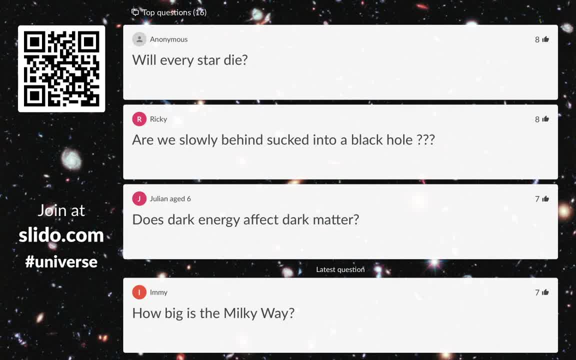 um, the answer, the answer is is yes, which is a slightly depressing question, sorry, a slightly depressing answer, but the answer really is yeah. um, all stars are burning fuel. that's how they make starlight and the heat from stars, and the answer is yes, and the answer is yes and the answer is: 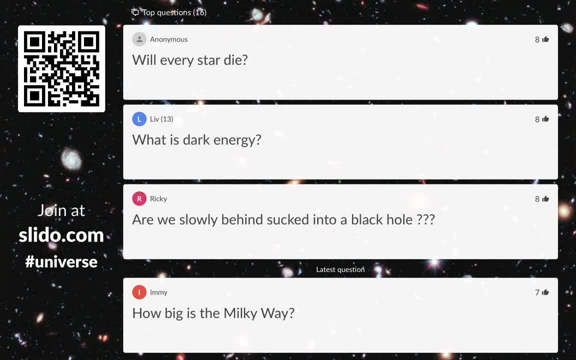 no, and eventually all the fuel will have run out. um, so the future of the universe really is black holes, and the black hole era of the universe, once all the stars have died, is going to go on for a much, much, much longer time than the kind of star era that we're living in now. so there might be.